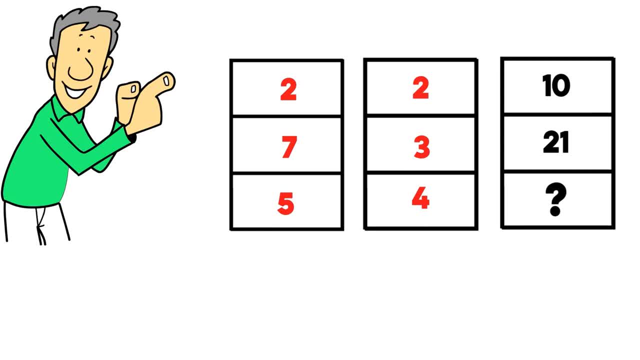 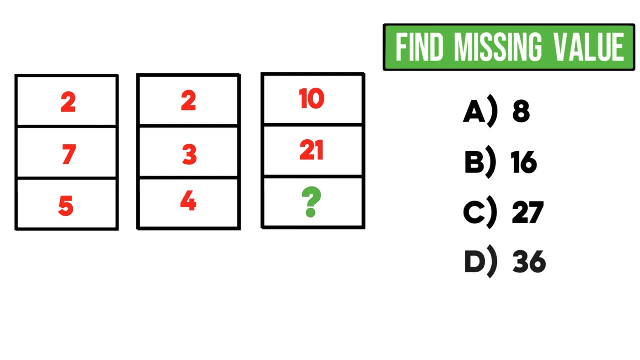 And in the last rightmost column, column number 3,, we see numbers 10, 21 and then one number missing. You need to find the missing value, which is highlighted by a question mark. You need to find the missing value and you have four choices to choose from: Choice: 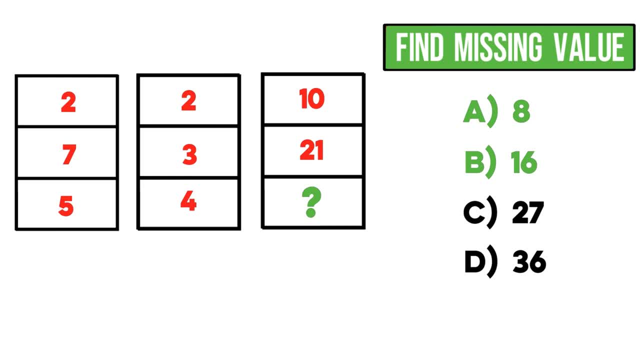 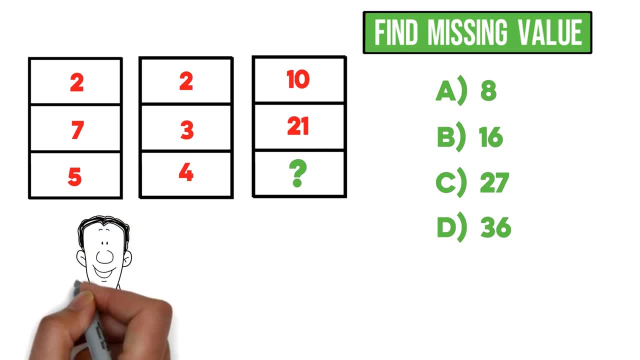 A – 8, choice B – 16,, choice C – 27 and choice D – 36.. Do you think you can recognize missing value? Give yourself 5 to 10 seconds to see if you can come up with the answer. 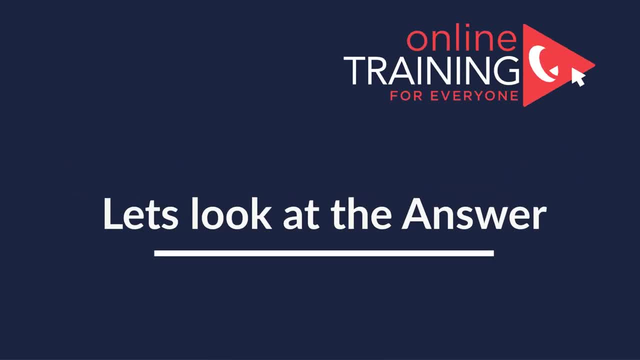 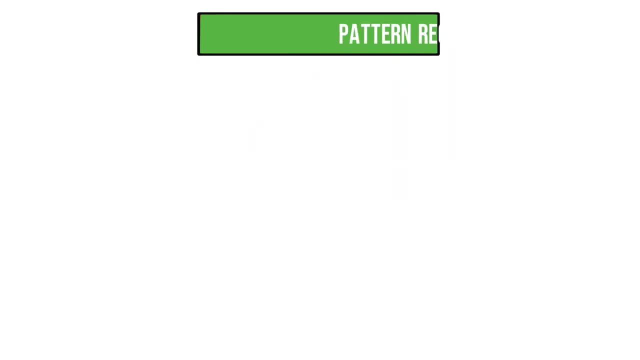 Did you figure out the solution? Let's continue to see how we can get to the correct solution together. The most important skills to solve these types of problems is pattern recognition skill. To recognize the pattern, you need to look closely into each column. Selective values. 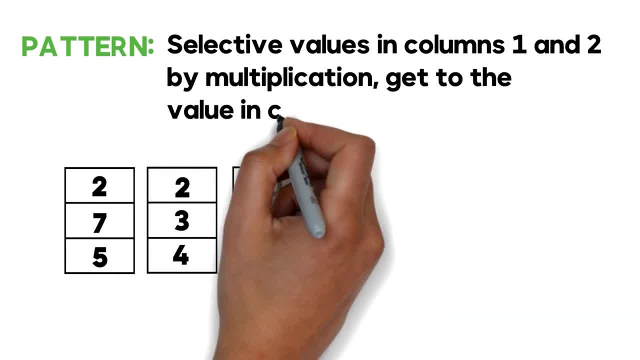 in columns 1 and 2 by multiplication get to the value in column 3.. And this is our pattern. Let's take a closer look for the values that are already present. If we multiply 5 by 2, by 9, then we will find that 6 is the correct value. Let's continue. 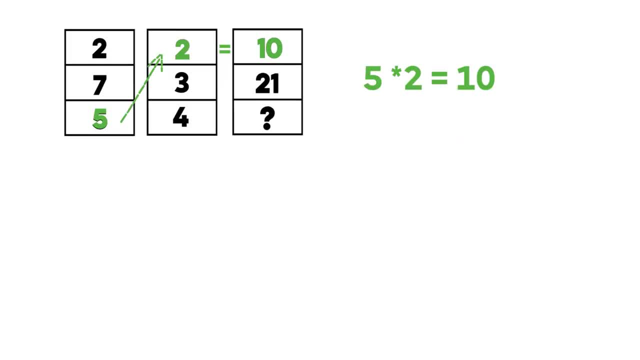 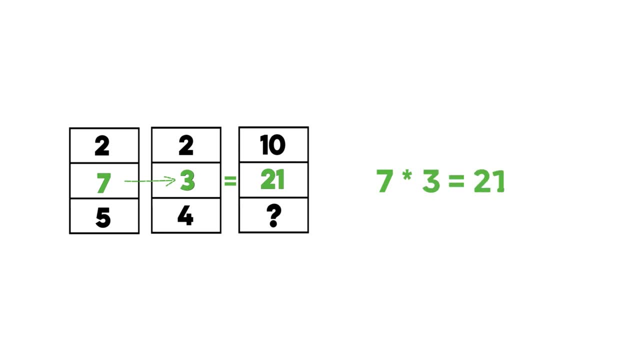 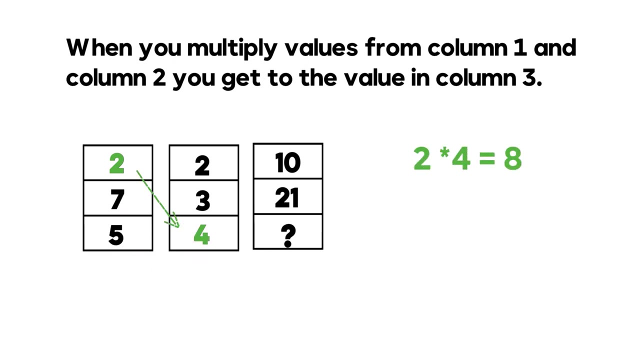 here 2, we get to the value of 10. second set of values represented by the middle row: 7 multiplied by 3 equals 21. so the missing values here can be calculated by multiplying 2 by 4 and the end result would be equal to 8.. so the correct answer to this problem is choice a 8.. i also wanted to 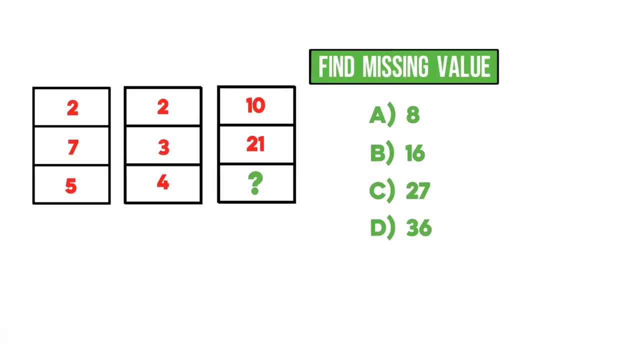 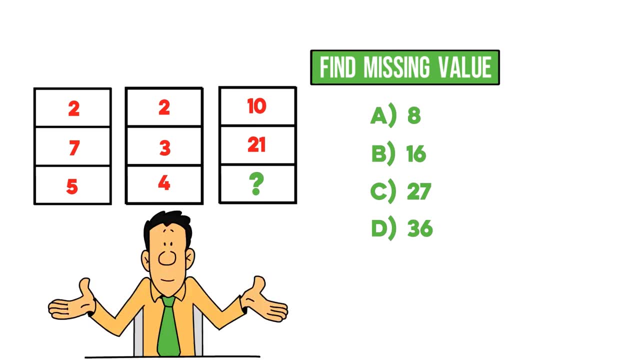 share with you one of the typical mistakes people make as part of answering these types of questions. people start looking at the columns themselves, but unfortunately there is no pattern just by looking in the values in column one, since pattern just doesn't exist if you look only at the values. 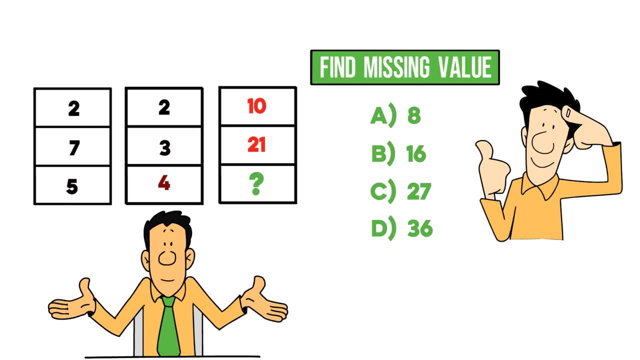 in column one or only at the values in column two or only at the values in column three? you will not be able to come up with the answer. you have to look across and take a global view across multiple columns to get to the correct solution. can you do me a favor if you have a better? 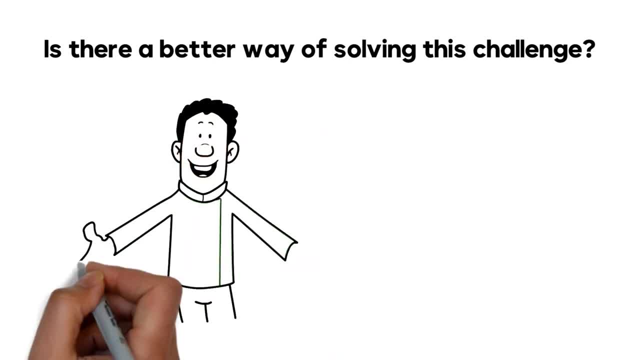 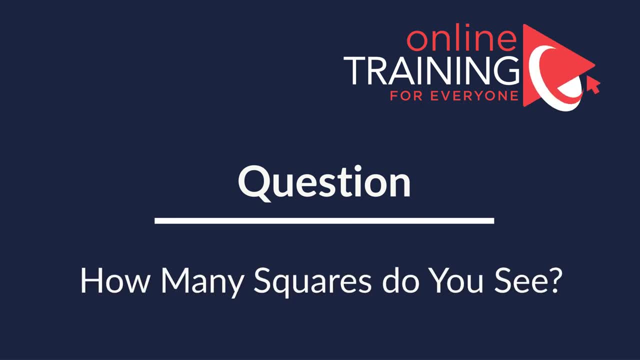 way of solving this challenge. please share your thought process in the comment section of this video. i'm very excited to share with you this question, which we frequently see on the test. despite being tricky, you will have a lot of fun trying to find the answer. this is one of those. 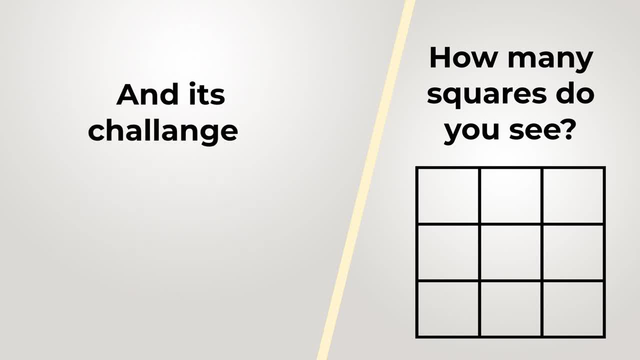 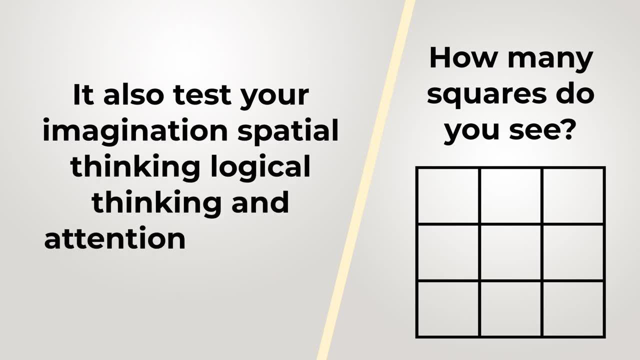 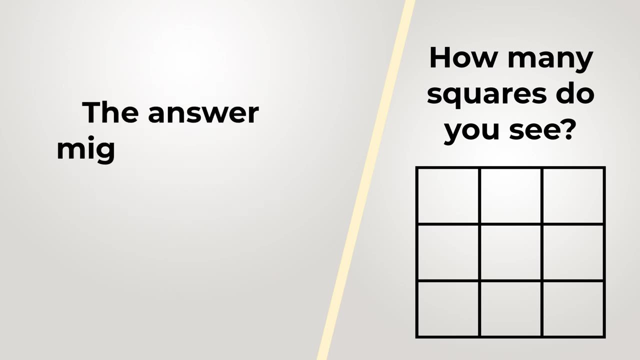 questions. that is easy to understand and it challenges your brain and improves your iq. it also tests your imagination, spatial thinking, logical thinking and attention to details. take a look at the picture and see: how many squares do you see? think again. the answer might be more challenging than you think. now might be the good time to pause this video to see if you can come. 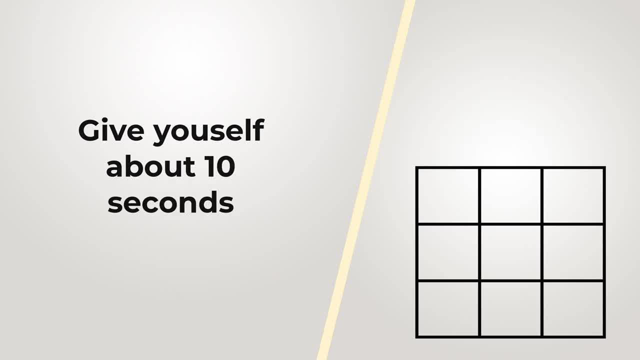 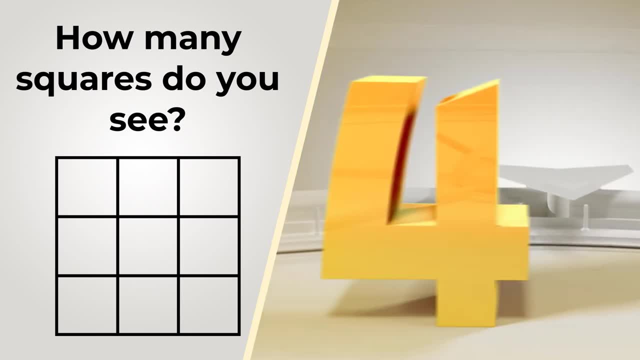 up with the answer on your own. give yourself about 10 seconds. this is typically how much you will get on the real test. do you know the answer? let me give you a tip. keep in mind, though, that on the real test, most of the time you don't get any tips. 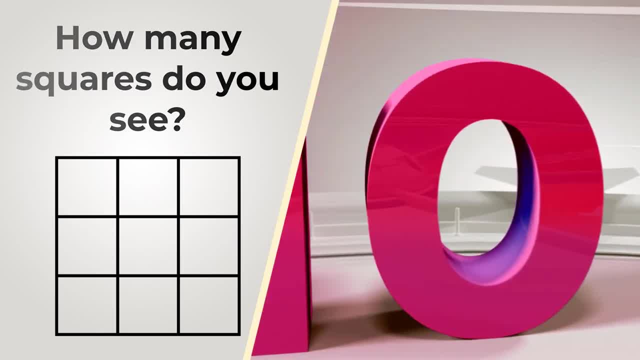 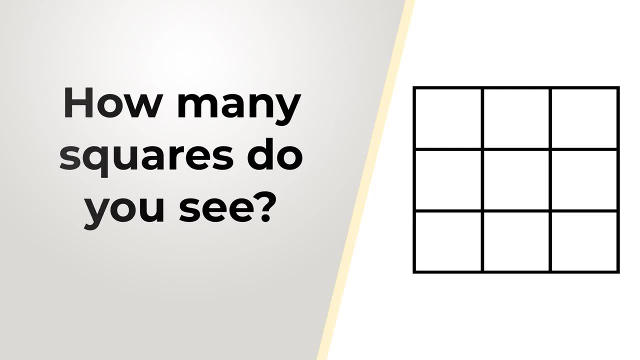 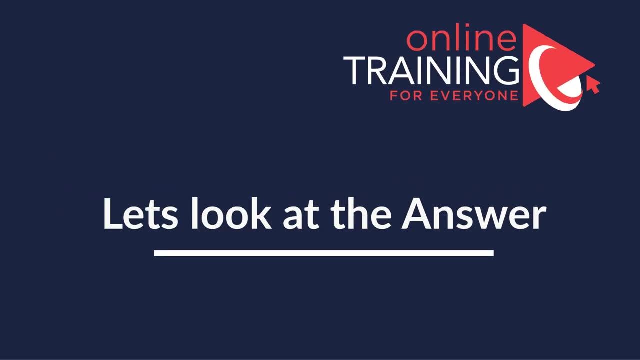 but since we're doing it together, i'd like you to consider the possibility of one shape being inside the other. let's continue to see how we can solve this challenge and get to the correct solution together. there are 14 squares that can be identified in this picture. this definitely came. 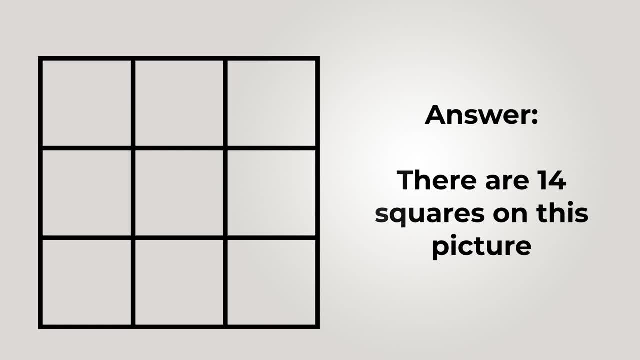 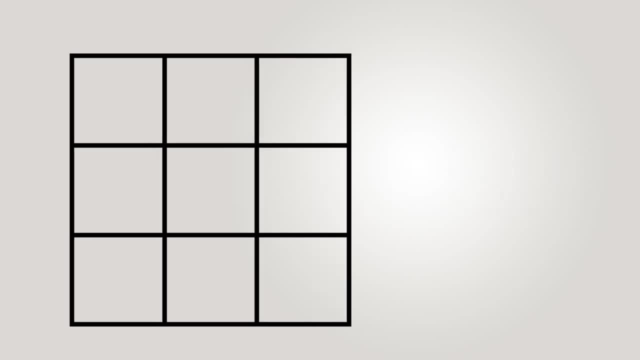 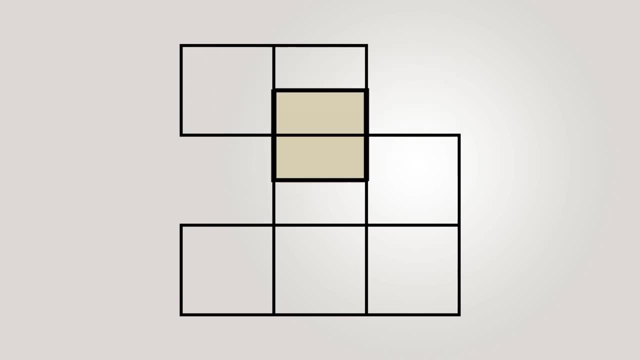 as a big surprise to me. do you see them all? some of them might be much easier to identify than others. let me draw them for you. there are nine small squares: one, two, three, four, five, six, seven, eight and nine. even though small squares are easy to see and identify, 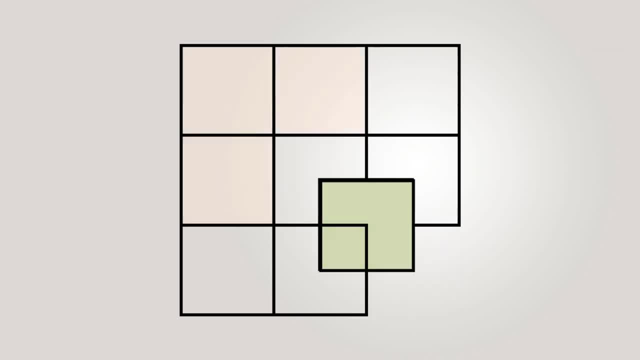 let's look at the medium-sized squares. there are four of them: number 10, number 11, number 12 and number 13, and then there is one large square. this is number 14.. what do you think about this challenge? were you able to solve it right away? 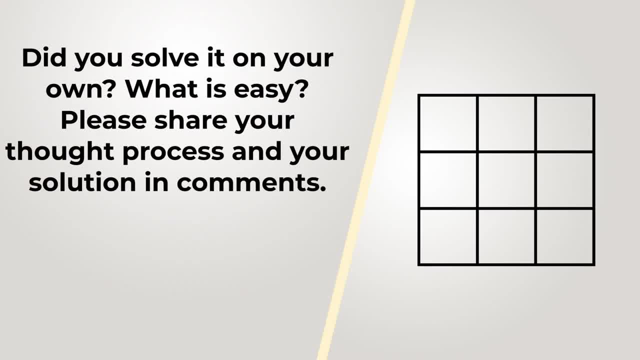 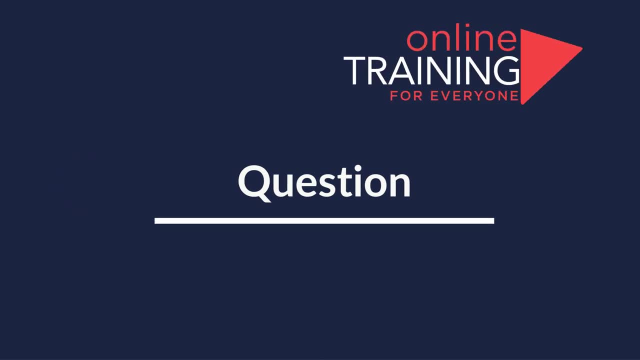 in case you see some additional shapes that we missed, which is always a possibility, please make sure to share them in the comments of this video. hopefully you've nailed this question and now know how to answer similar problems in your own language. problems in the test. I gotta tell you I love this question. This is such a unique question. 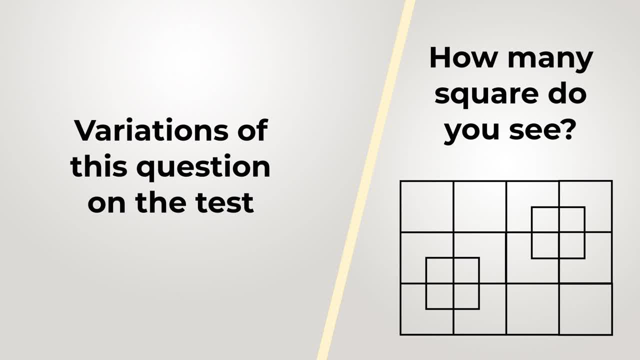 and we see a lot of variations of this question in the test. In this particular version, you are presented with the 4x3 matrix of squares and then you see two additional squares on top of the medium-sized squares And the question is: how many squares do you see on the picture? Take a closer. 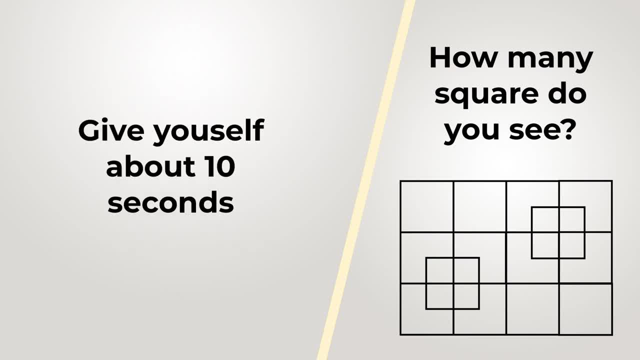 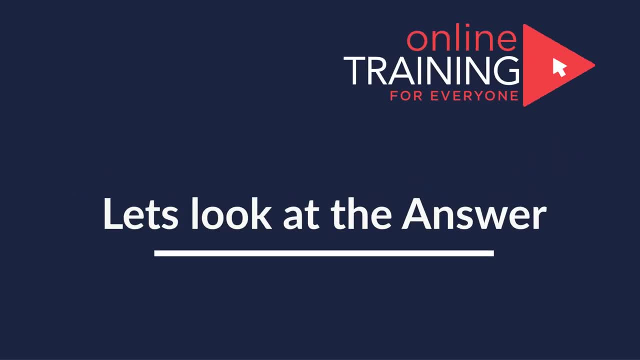 look and give yourself a little bit of time to find out the answer. Feel free to pause this video if you need more time. Do you have the answer? Let's continue to see if we can come up with the solution together. As you might have figured out, there is a total of 30 squares shown in this. 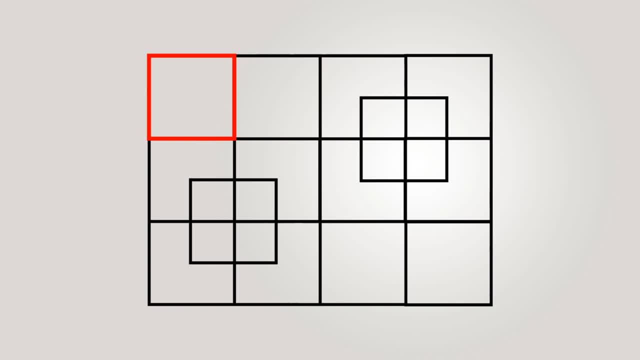 picture. Let's start by removing overlapping squares and counting medium-sized squares. There are 12 of them in this picture. Let me count them all for you: 1,, 2,, 3,, 4,, 5,, 6,. 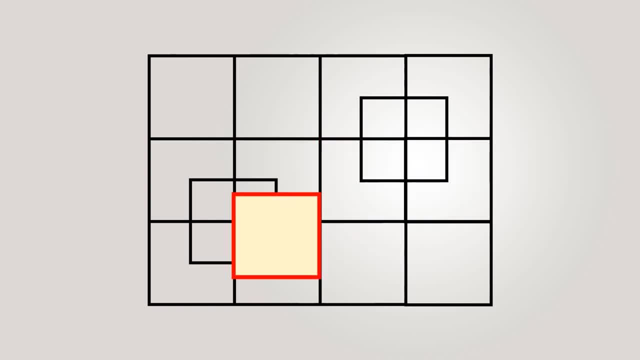 7,, 8,, 9,, 10,, 11, and 12.. Once we reintroduce overlapping squares, we can count them as well. They would have numbers 13 and 14.. Two overlapping squares introduce eight small squares. 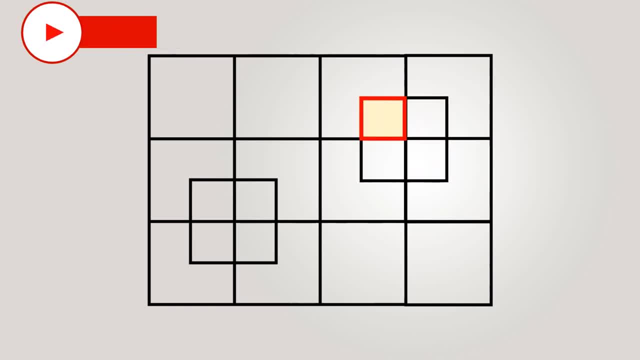 They would have numbers 15,, 16,, 17,, 18,, 19,, 20,, 21, and 22.. There are also six large squares. Let's give them a number: 23,, 24,, 25,. 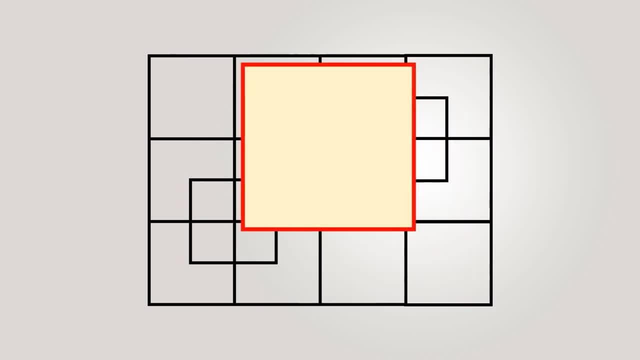 26,, 27,, 27, and 28.. As you can see, those large squares are located in the top row as well as in the bottom row. And, last but not least, are two extra large squares. I gave them the numbers 29 and 30.. 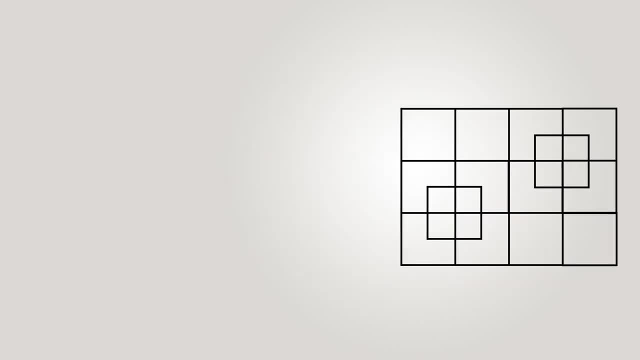 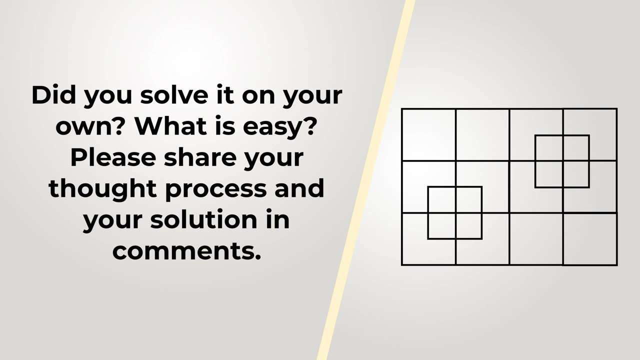 Were you able to solve this challenge on your own? Did you get to the right answer, Or maybe we missed some of the squares? Feel free to share this information in comments, and I hope this question was nailed by you and now you know how to answer similar questions on the test. 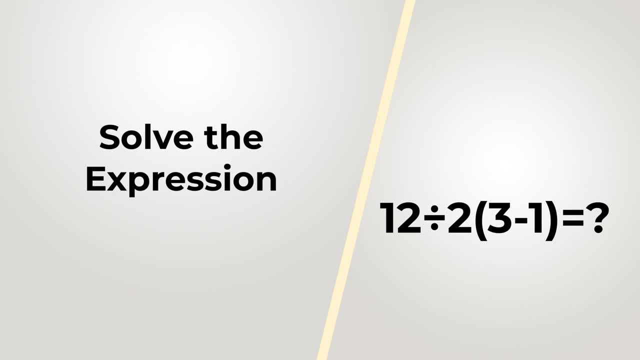 Here's the interesting question, which is easy to understand but at the same time you will have a lot of fun solving it. You need to calculate the simple expression 12 divided by 2 and then multiply it on the value in parentheses, which is 3 minus 1.. Take a look closely and see if you can. 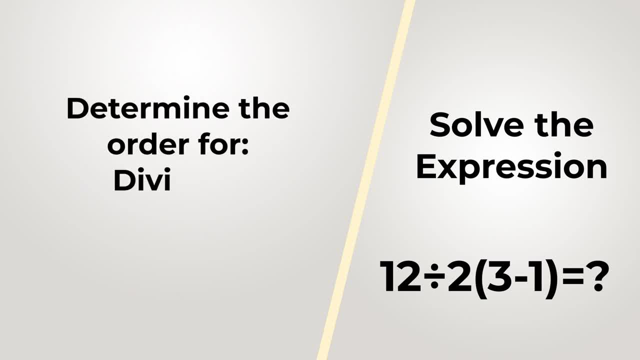 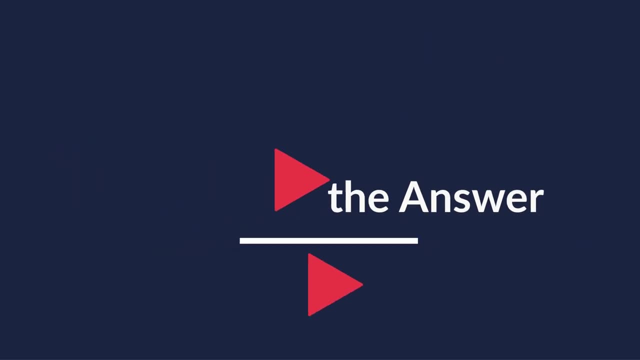 come up with the answer. There are three operations you can do to solve this question Here: division, multiplication and subtraction. All you need to determine is which one to do: first, second and third. Do you think you know the answer? Let's continue and get it solved together. 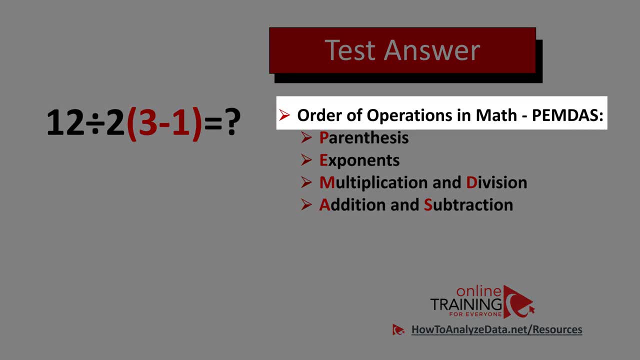 The order of operations in math tells us that the first expression we need to solve is in parentheses. We first need to calculate 3 minus 1.. And obviously the answer is 2.. The big question: what do we do next? The order PAMDAS tells us that we need to do multiplication and division. 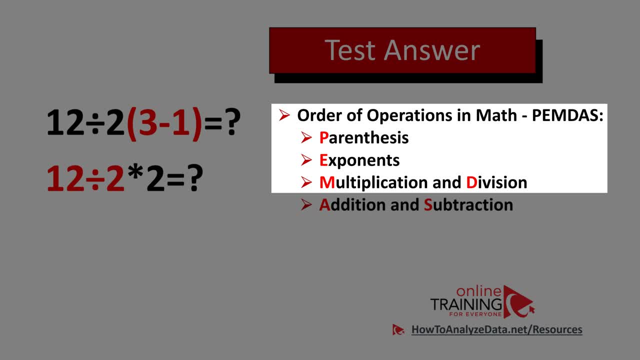 But what order doesn't mention is that we need to do it from left to right. And, what's interesting, the acronym itself is a little bit confusing, because it shows multiplication first and then division. But in our case we need to do division first. 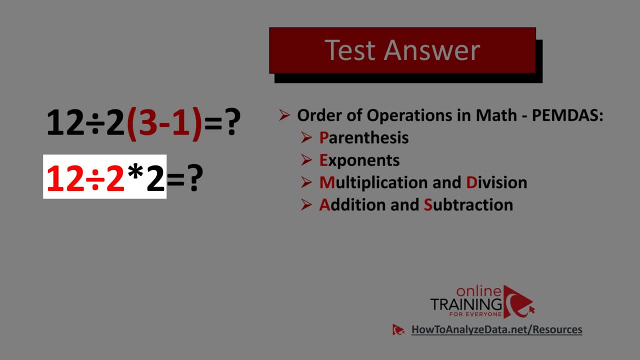 and divide 12 by 2 and then do multiplication. Once we divide 12 by 2, we get to 6 and the final number is 12.. So we need to divide 12 by 2 and then do multiplication, And we need to do this. 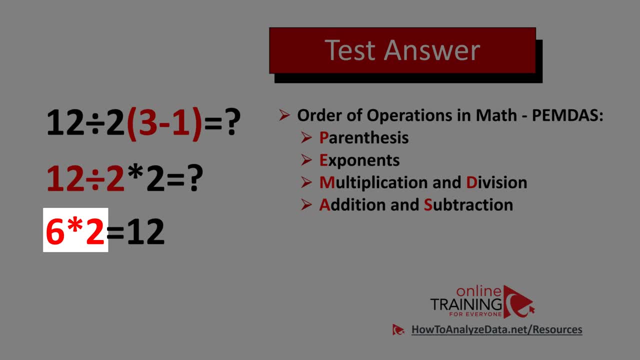 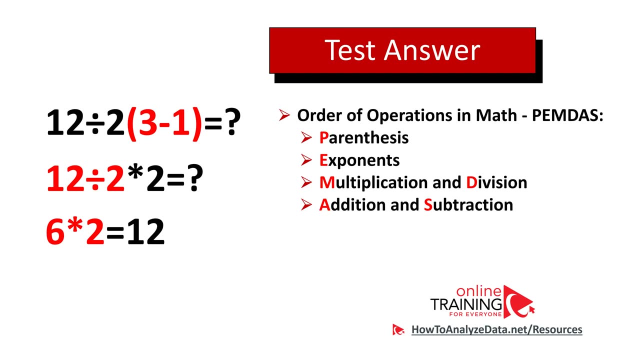 expression we need to solve would be 6 multiplied by 2, so the correct answer here is 12.. let me give you a quick hint. even if you don't know the answer, you can always use a calculator. most modern calculators do support expressions. let me demonstrate for example. if you type calculator: 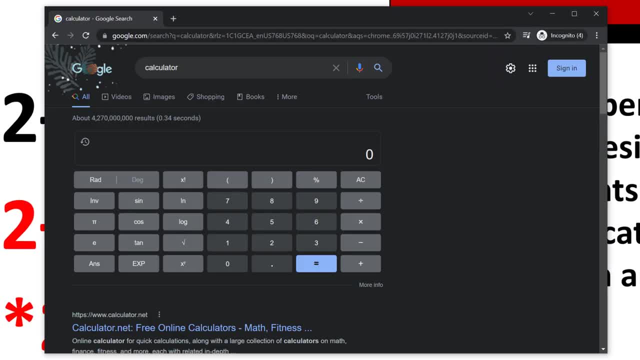 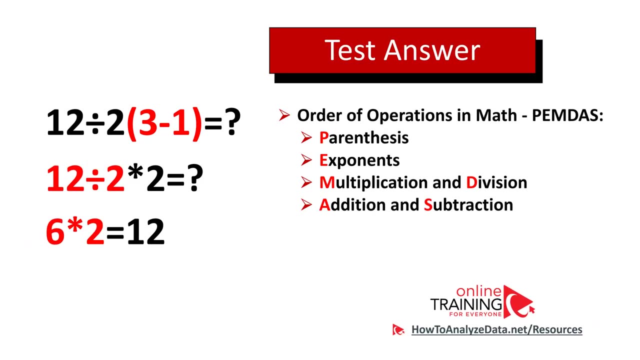 in google. it shows the calculator which you can use to solve the expressions. you can preview expression and once you hit the equal sign, it calculates it for you and you can see that the correct answer here is 12.. another alternative is to use microsoft excel, which is available. 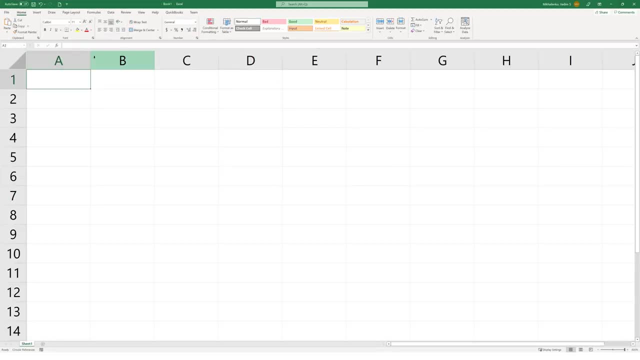 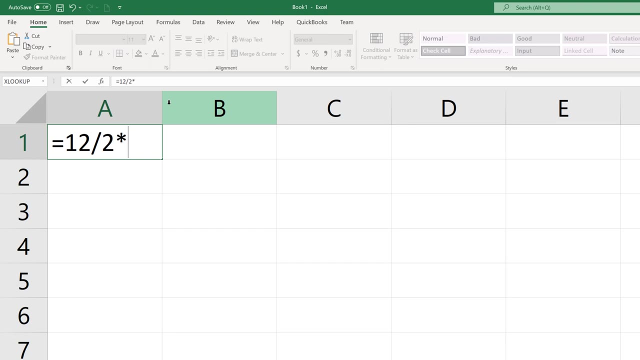 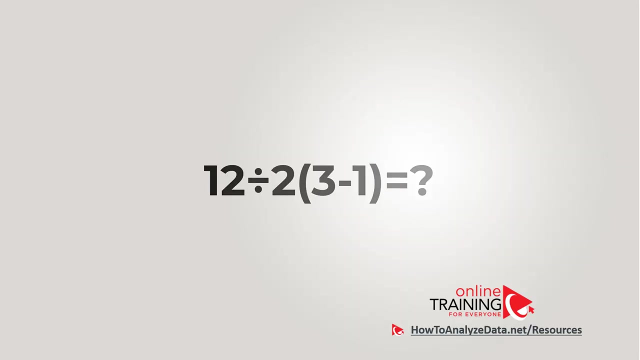 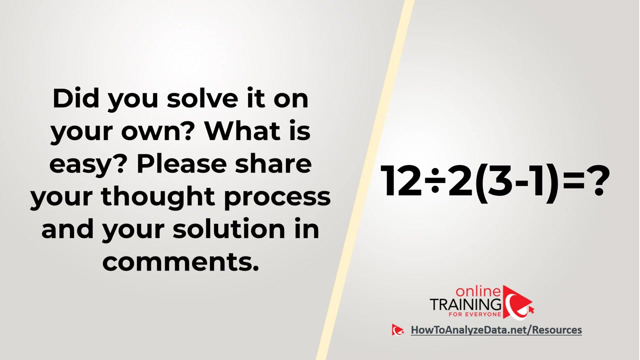 on almost any windows machine. here you can enter the expression right inside any cell and microsoft excel will perform the calculations. so did you solve this challenge on your own? was it easy for you? please share your thought process and your solution in the comment section of this video. 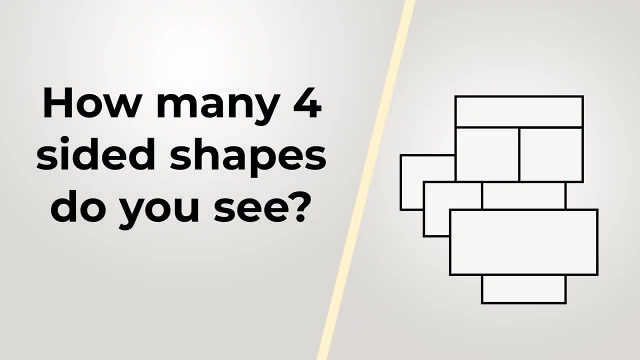 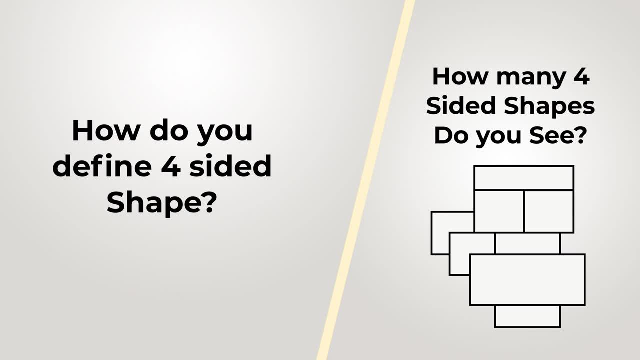 here is an interesting question which tests your spatial thinking. how many four-sided shapes do you see? and you're presented with the picture on the left which has a lot of different shapes. first, you need to be clear on the definition of four-sided shape and have a good understanding of what it means. 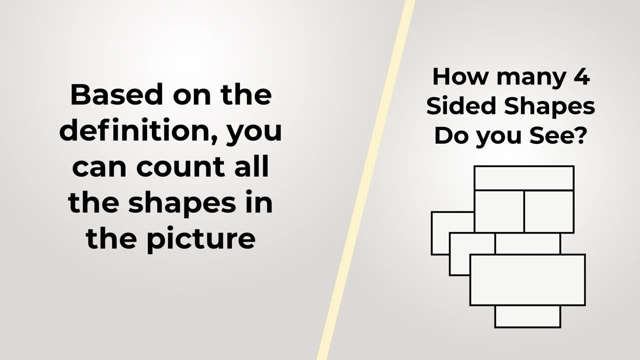 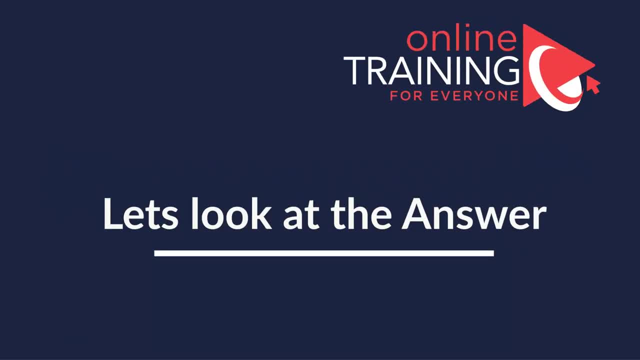 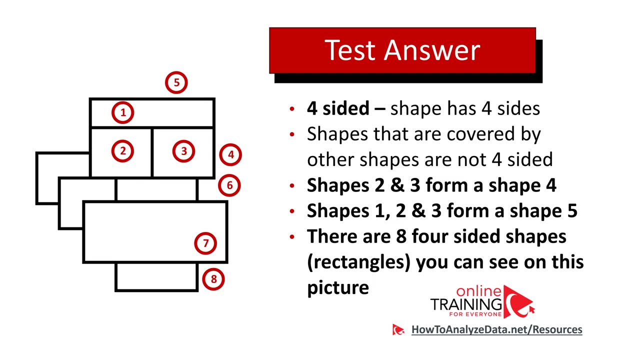 once you have the definition, you can count all the shapes on the picture that match this criteria. did you figure it out? let's jump to the solution so we can solve this challenge and get to the correct solution together. so, as i mentioned, first let's do a definition. 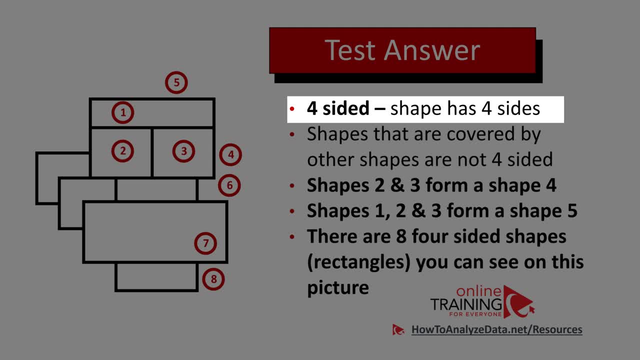 of the four-sided shape and the simple definition is that the shape has four sides. for example, rectangle has four sides, and you see a rectangle one here which has four sides, and this shape here matches the criteria. shapes that are covered by other shapes are not four sided. for example, we have something that mimics square here, but because it's covered by another. 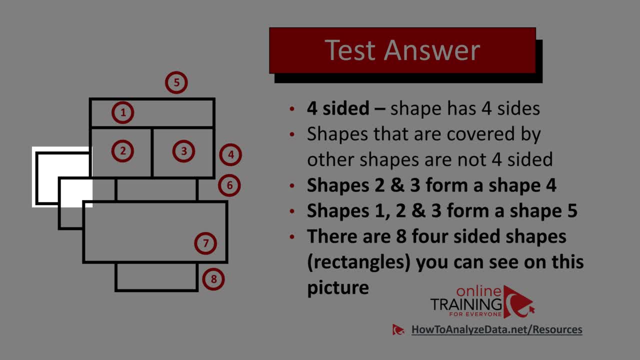 square. it is not four-sided. actually it has five sides. the key to answering this question is to make sure that you didn't miss any shapes. in fact, it's so easy to solve because there are seven. In fact, it's so easy to miss because some shapes are inside of the other. 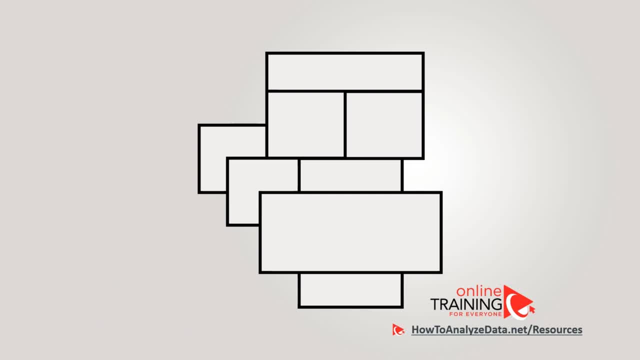 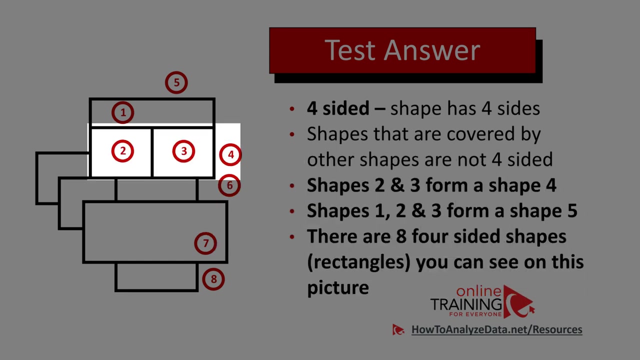 Let me show you all 8 shapes here on this picture: 1,, 2,, 3,, 4,, 5,, 6,, 7, and 8.. Let's look at inside shapes that form another shape, Shape 2 and 3 form shape 4.. 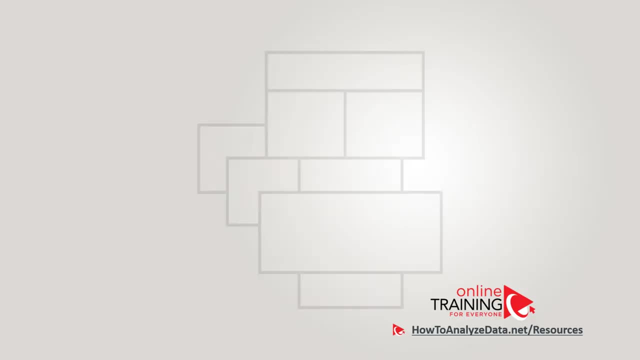 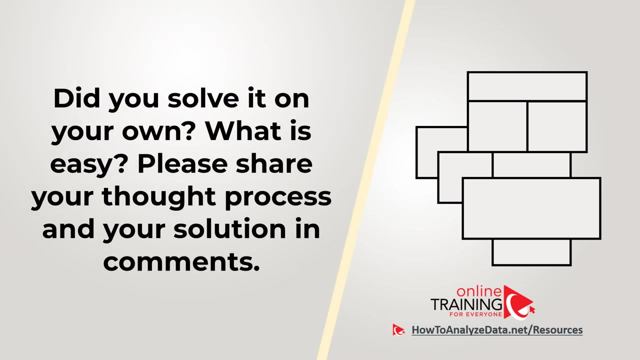 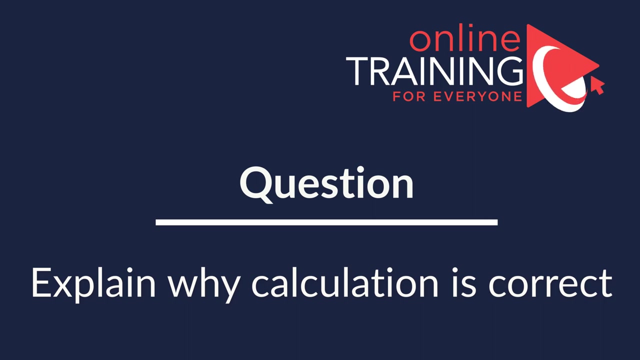 And shapes 1,, 2, and 3 form a shape 5.. Now was it easy to solve for you. Do you see any shapes we might have missed? Please share your thoughts in the comment section of this video. Here's the interesting question that might get you puzzled. 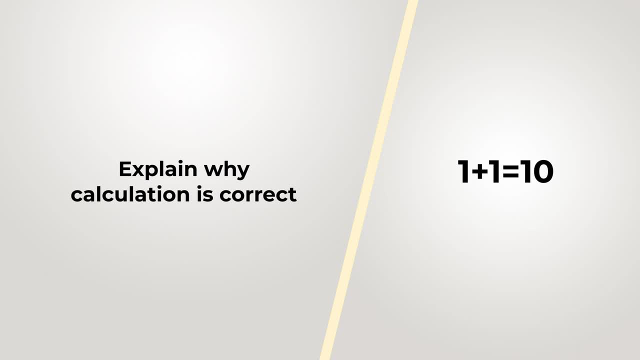 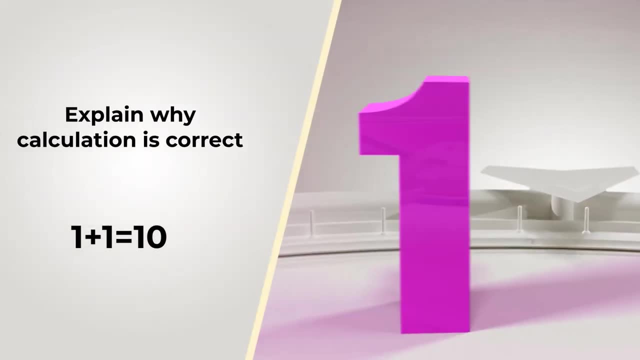 You need to explain why the calculations that you see is correct And you have a calculation: 1 plus 1 equals 10.. Give yourself 10 seconds And let me give you a hint: Try to think out of the box. 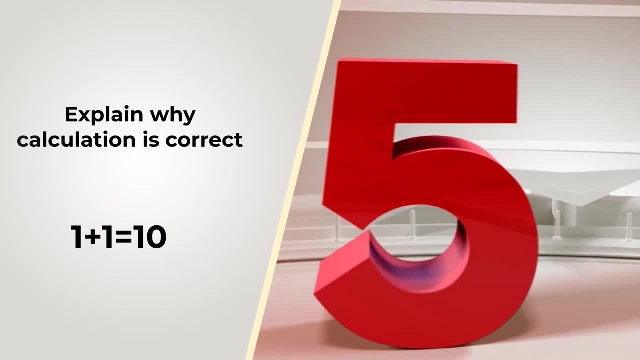 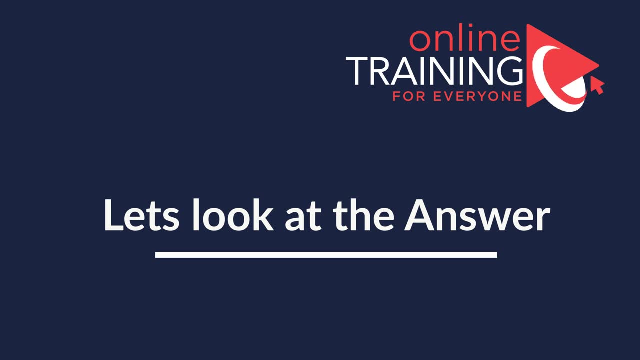 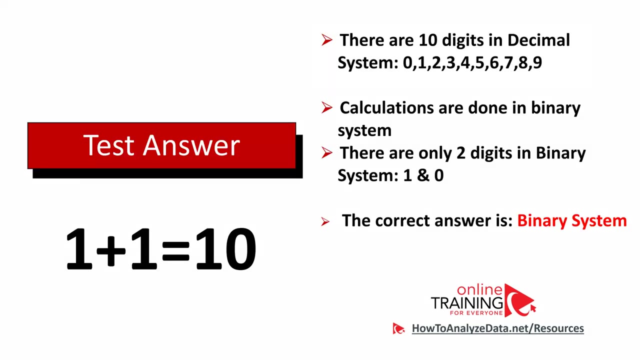 And try to see what else can be going on here besides just the calculations. Do you think you know the answer? Let's continue to see how we can solve this challenge and get to the correct solution together. Typically when we do calculations, 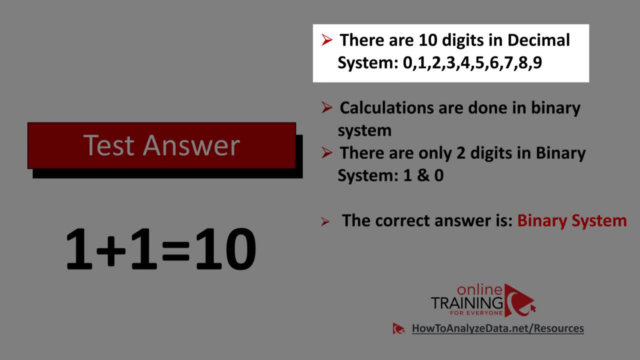 we use 10 digits. in the decimal system We use 0,, 1,, 2,, 3,, 4,, 5,, 6,, 7,, 8, and 9.. But here calculations are done in a binary system. 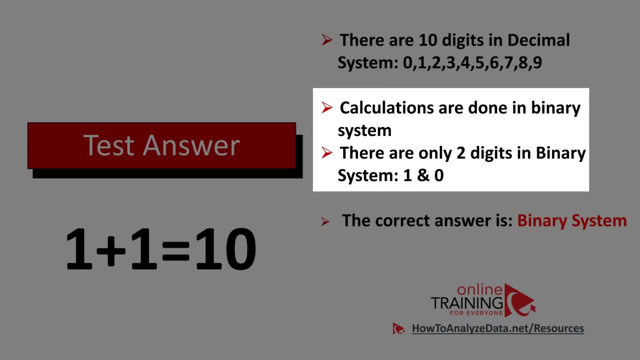 And there are only two digits in the binary system: 1 and 0.. So what happens when you get a calculation in the binary system and you add 1 plus 1?? What looks 10 in the decimal system looks like 2 in the binary system. 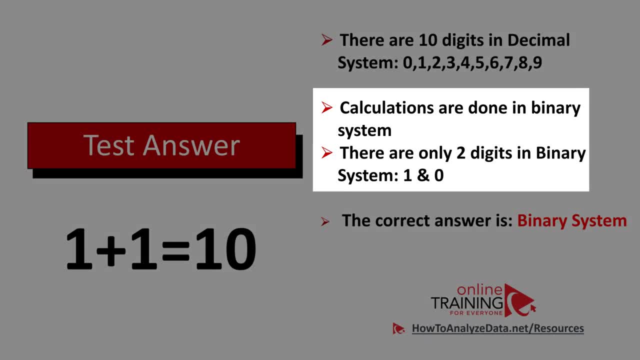 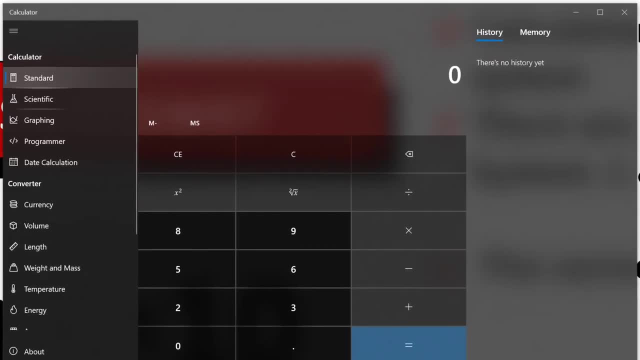 So the correct answer. this calculation is possible because of the binary system. Let me demonstrate this to you. If you launch Calculator in Windows and then switch to the Programmer Calculator, you can choose different systems. By default, it's a decimal system. 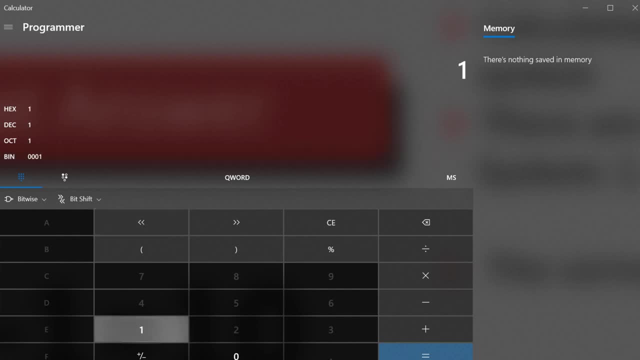 But if we switch to binary and then we can add, 1 plus 1 equals what looks like 10. in reality is 2 in the binary system. Hopefully you've nailed this question and now know how to answer similar problems. 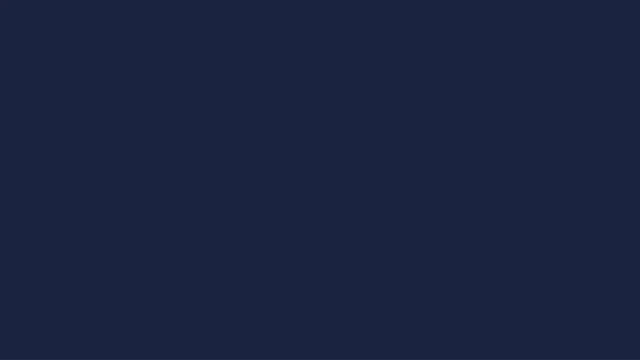 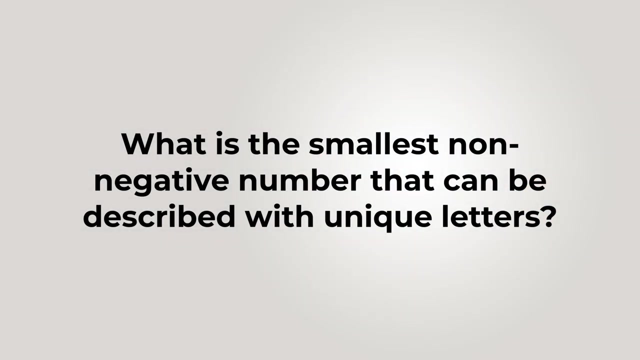 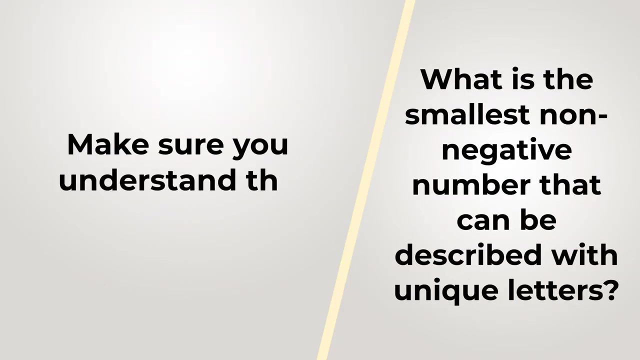 on the test. Here's the challenging question you might frequently see: on the test: What is the smallest non-negative number that can be described with unique letters? You might have to re-read this question multiple times just to understand what is being asked. 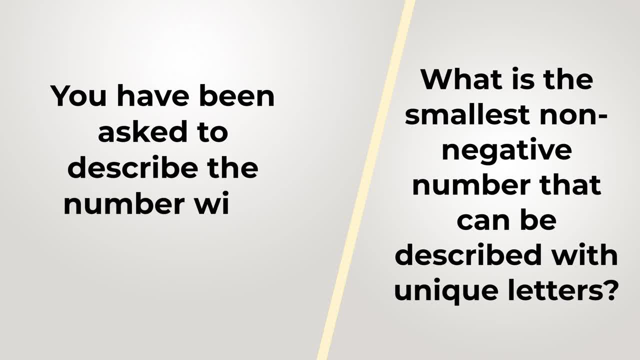 Let me help you If we are to clarify this question. you are being asked to describe the number with the letters, And those letters should be unique. For example, in the word 20, there are two letters, T, So 20 is not the word that can be used in the test. 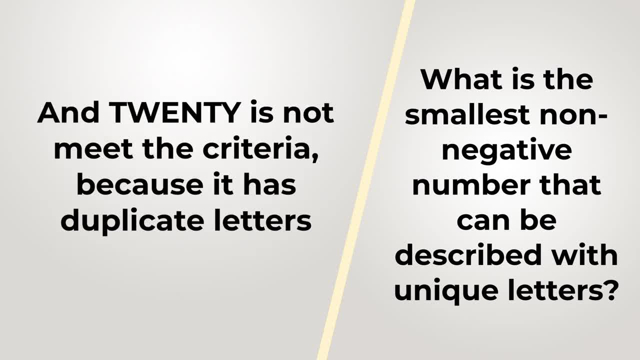 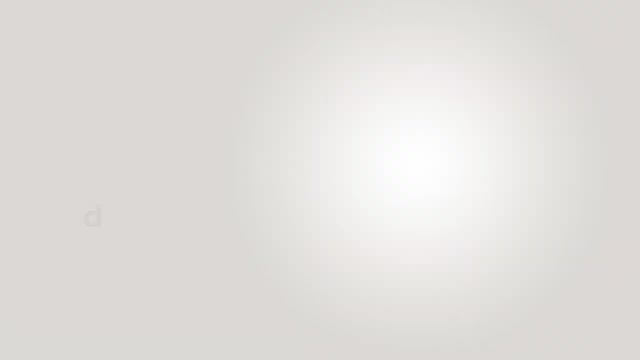 On the other hand, so, which means that 20 is not the word that meets the criteria because it has duplicate letters. On the other hand, word 10 contains all unique letters. So the question is: what is the smallest non-negative number? 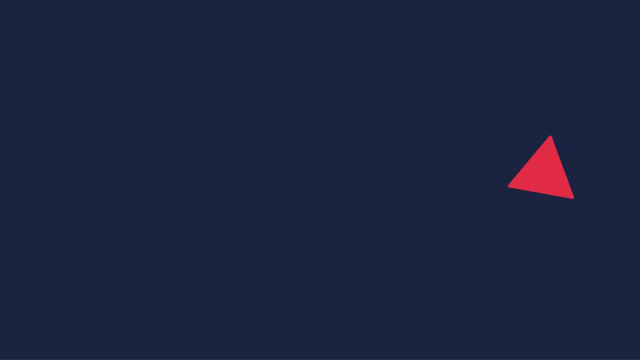 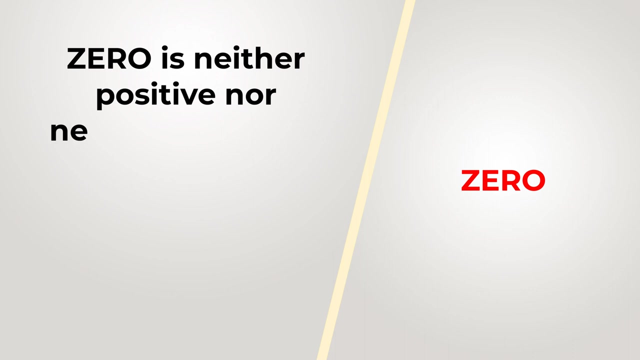 that can be described with unique letters. A lot of times people get the answer 1. and this might be true because 1 is the positive and all letters are unique, But the actual answer to this question is 0.. 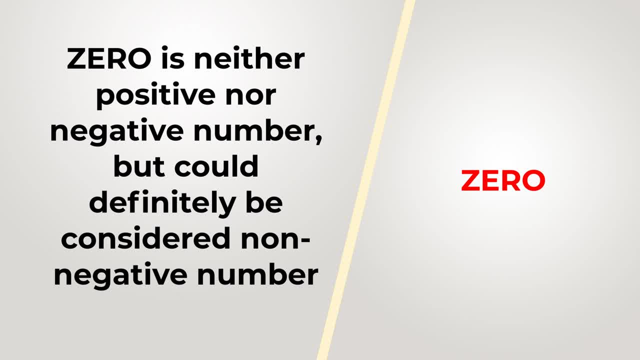 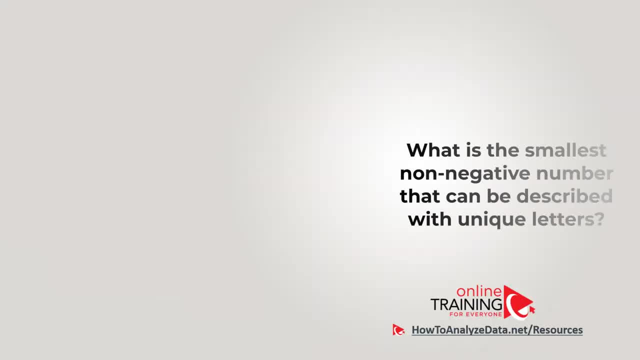 because 0 is neither positive nor negative number, but can definitely be considered as a non-negative number. So the correct answer here is 0.. Did you figure it out? Please share your thoughts and the way you approach this question. 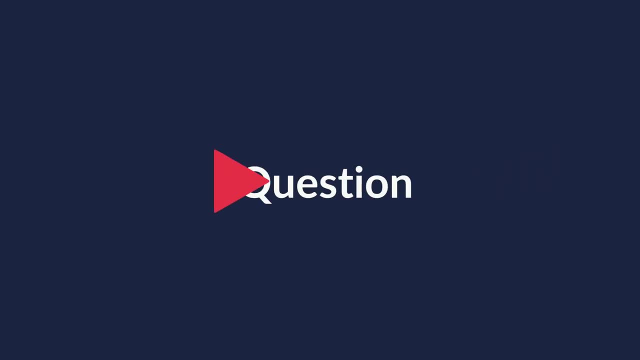 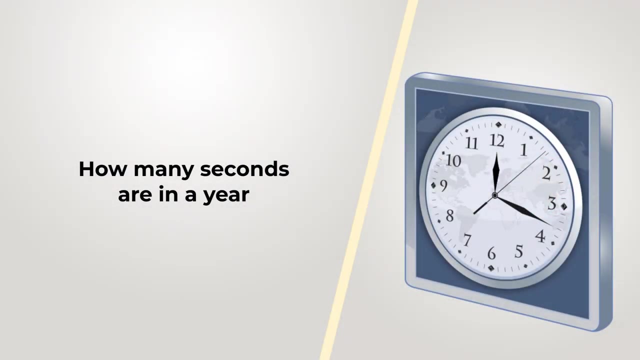 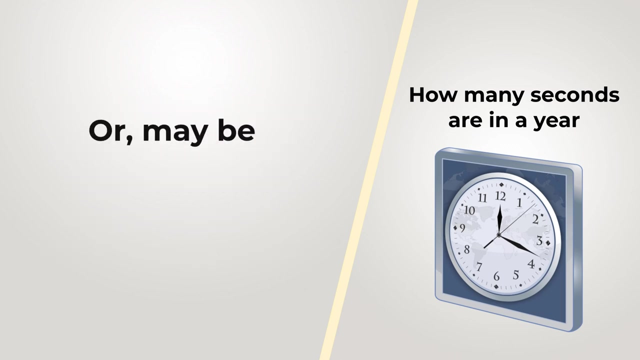 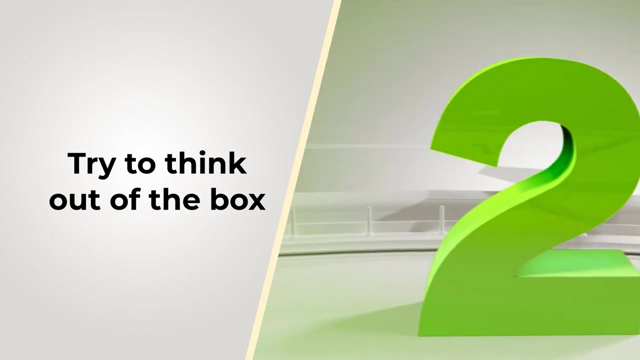 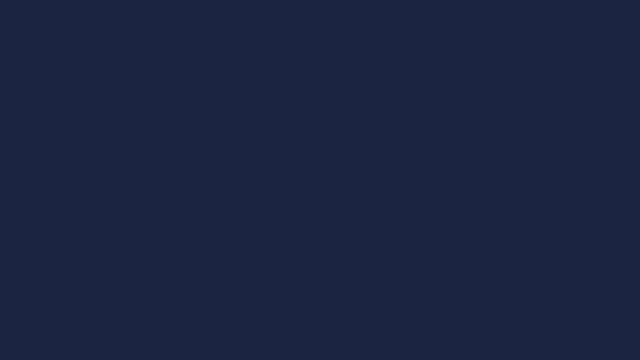 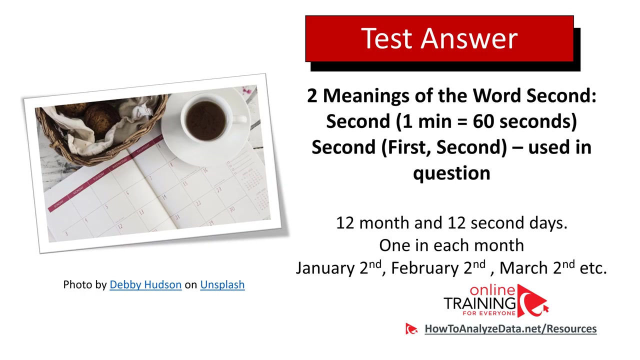 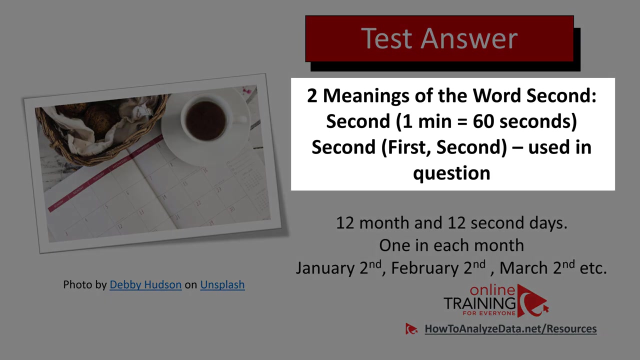 in the comment section of this video. Thank you very much for watching this video. See you in the next video. Thank you very much for watching this video. There are 12 months and there are 12 second days. one second day in each month. 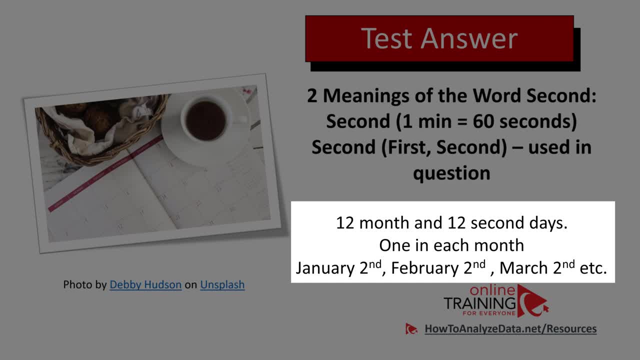 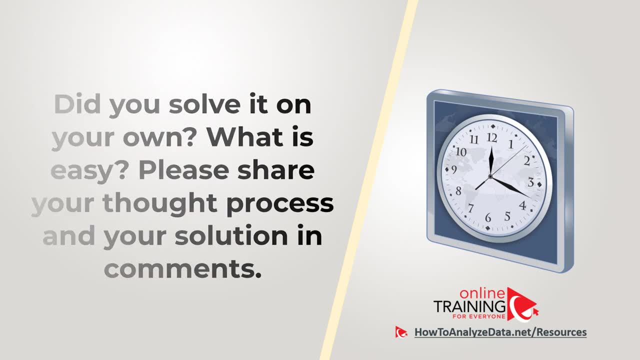 January 2nd, February 2nd, March 2nd and etc. Hopefully you've nailed this question. it gives you some laughs and you now know how to answer similar problems on the test. This is one of my favorite questions. 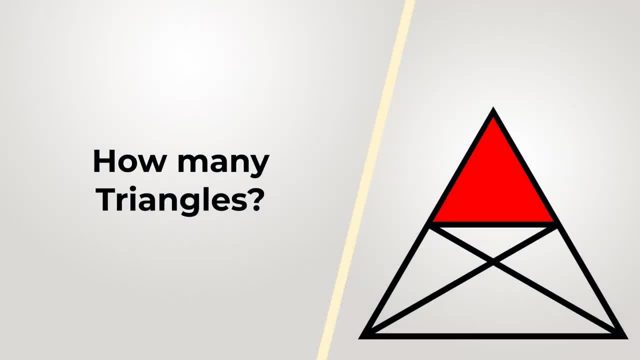 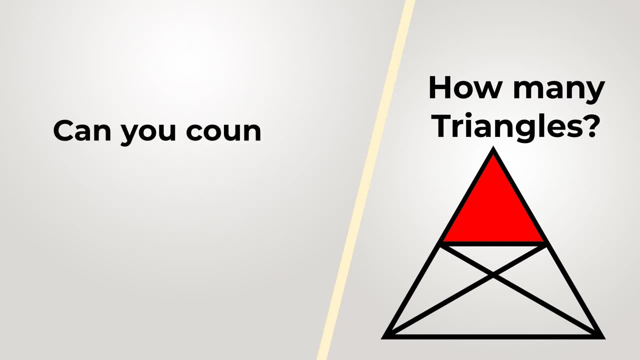 and there is a very high chance that you will get it on the assessment test. How many triangles do you see? The answer is presented with the shape. on the left, There are large triangles and there are also lines inside of these large triangles. 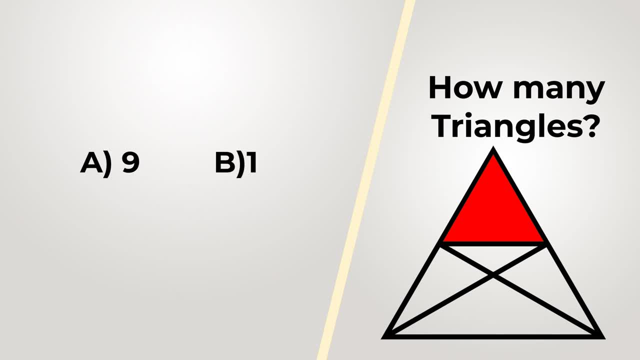 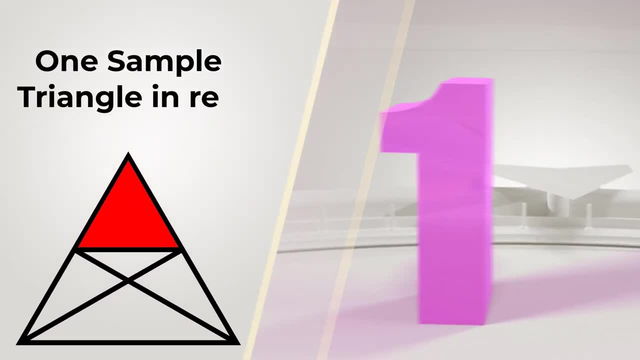 You have four different choices: Choice A: 9 triangles. choice B: 12. choice C: 17. and choice D: 24. One triangle is highlighted in red, but there are a lot of other triangles. 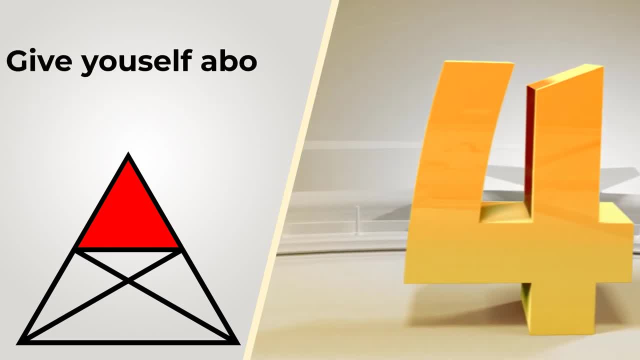 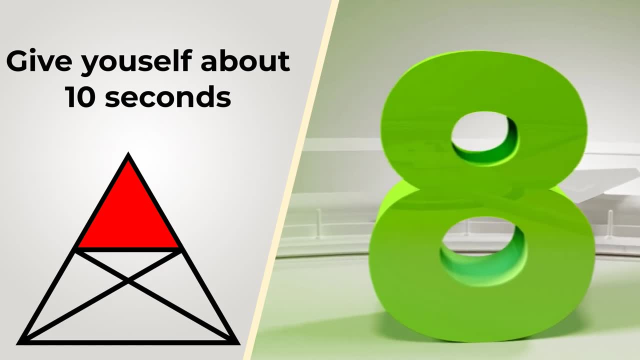 Do you think you know the answer? Give yourself a few seconds. I would recommend 10 to 15 seconds. This is about as much time as you will get in the real test. You can pause this video to give yourself some time to figure out the answer. 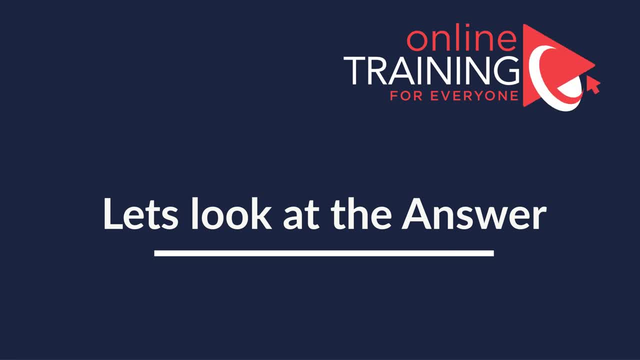 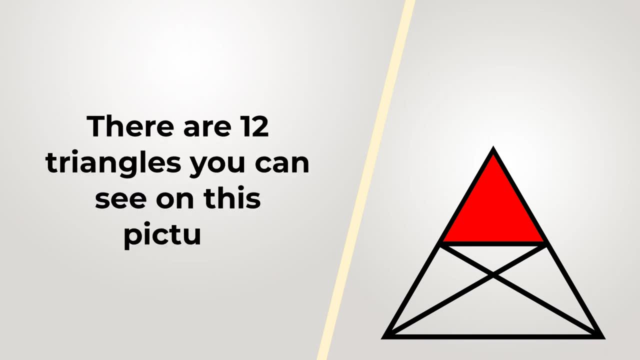 I am going to continue and reveal the correct solution so we can get to the answer together. I counted 12 triangles in this picture. Is this what you got too? Let me show them all for you. I'll start with the smaller triangles. 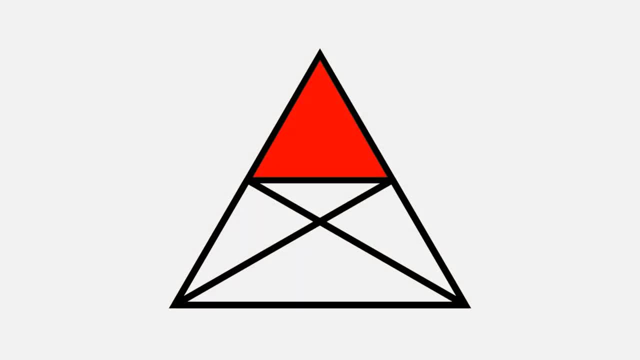 and then go to the medium-sized ones and then go to the large ones: One, two, three, four, five, six, seven, eight, nine, ten, eleven. 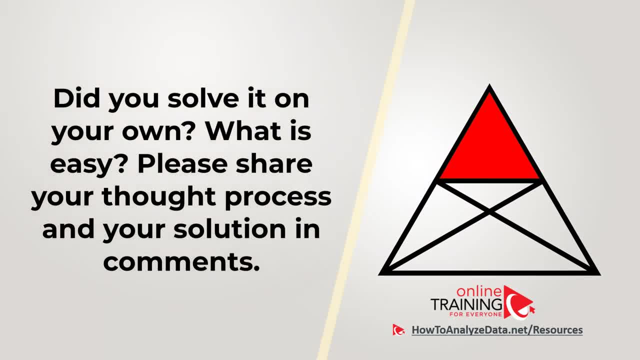 and twelve Did you come up with the different answer? Please share your thought process in the comment section of this video so we can all learn from your perspective. Hopefully, you nailed this question and got to the correct answer on your own. 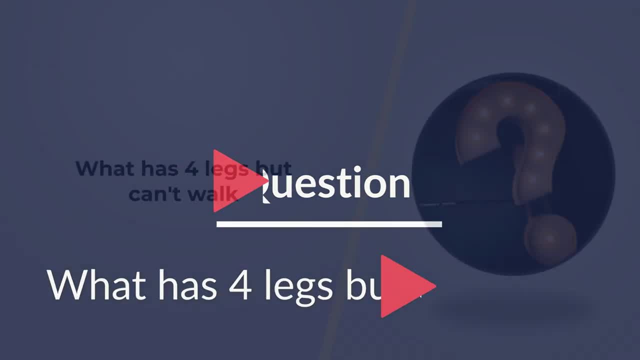 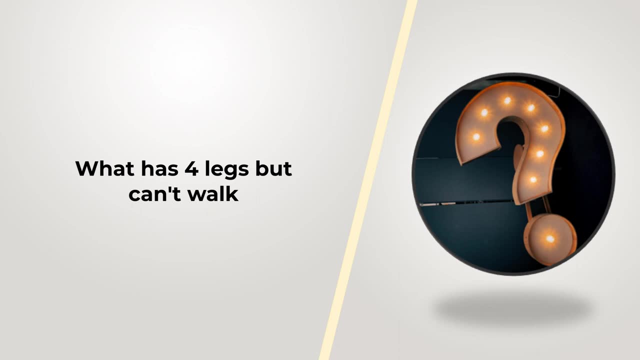 Here is the question which tests your understanding of English language, your vocabulary as well as your ability in logical reasoning: What has four legs but can't walk? Do you think you know the answer? Now might be a good time to pause this video. 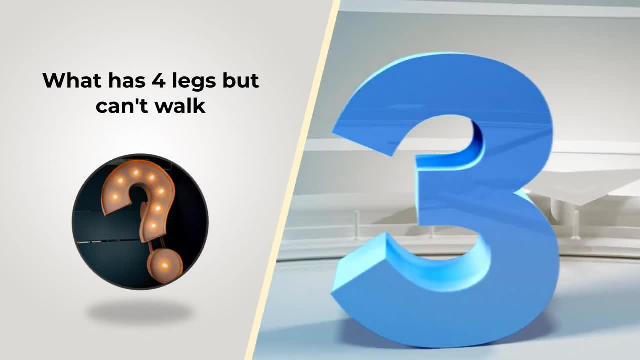 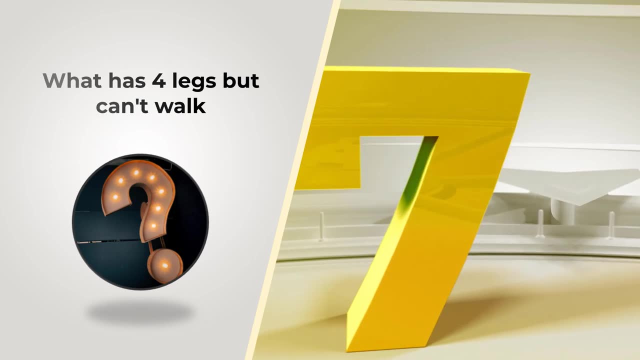 to see if you can come up with the answer. Do you think you found the answer? Let me give you a quick hint: Think out of the box and think of not necessarily something that walks. Did you figure it out? Let's continue. 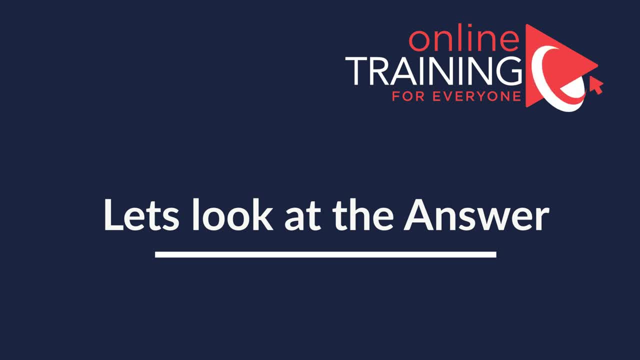 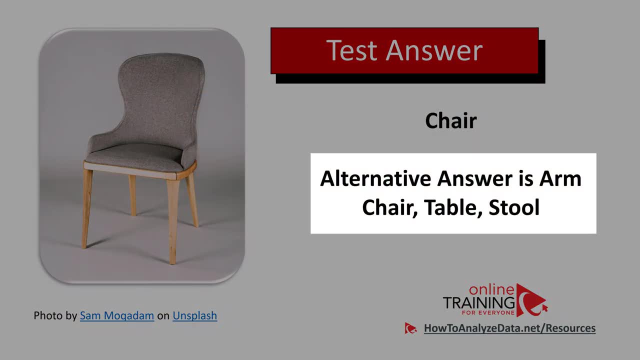 to see how we can solve this challenge and get to the correct solution together. As you might have figured it, the answer is chair And the alternative answer could be armchair, table or stool. Hopefully, you figured it out on your own. 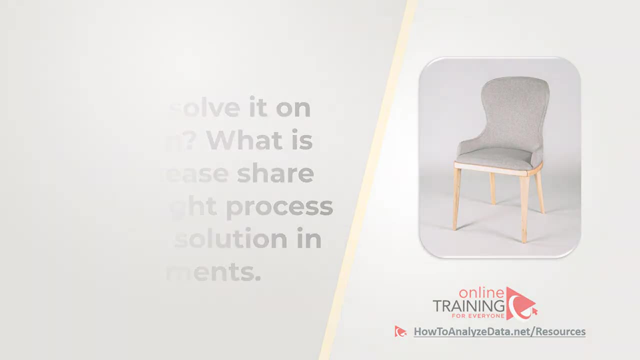 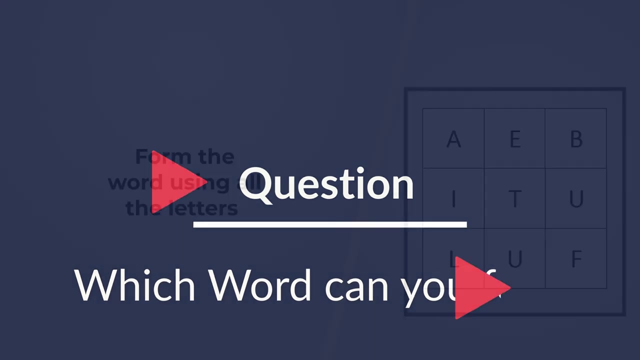 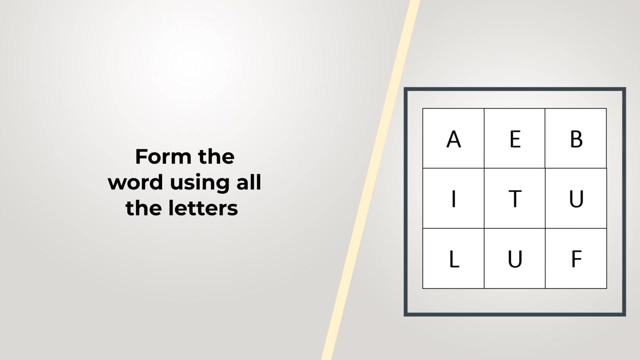 and now know how to answer similar problems on the test. Here is the tricky question which tests your imagination without using the words and logical reasoning. What word can you form using all the letters in the box? 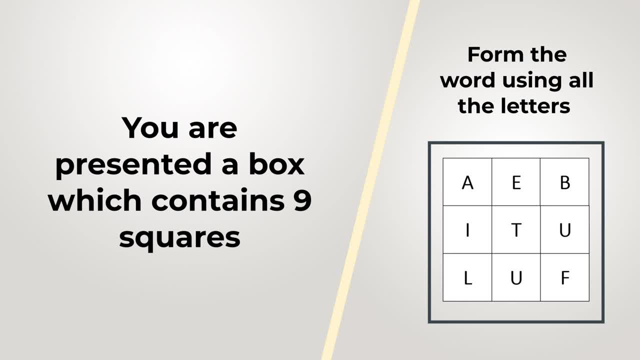 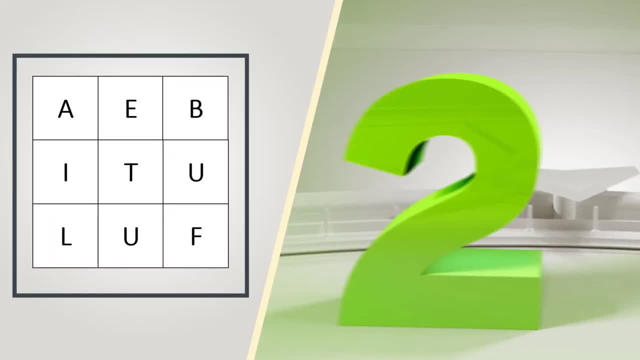 And you are presented with the box that contains nine squares and each square has a letter inside. Take a closer look at this picture and see if you can come up with the answer. This might be the right time to pause this video. 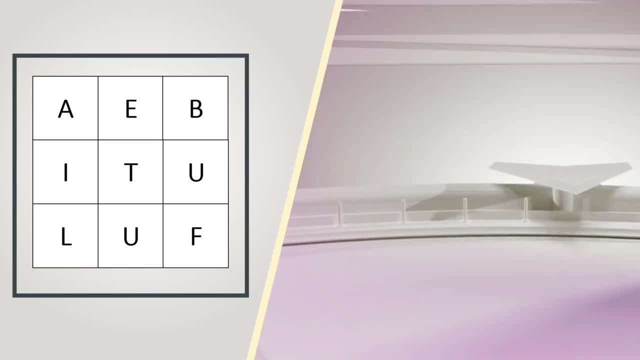 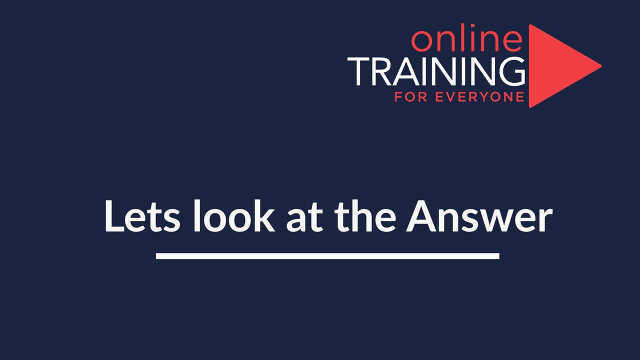 to see if you can come up with the answer on your own. Do you think you know the answer? Let's continue to see how we can solve this and get to the correct solution together. Obviously, there are quite a few words. 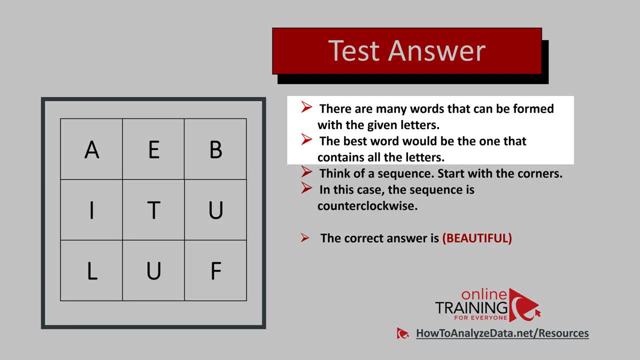 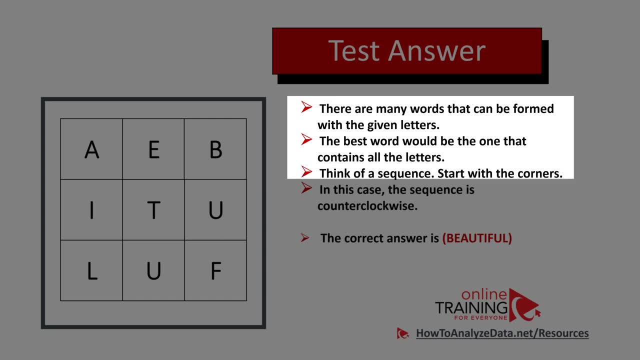 that can be formed with these letters. But the best word will only contain one of each of the nine letters presented here on the screen. The best solution here is think of the sequence A lot of times. authors of this question. 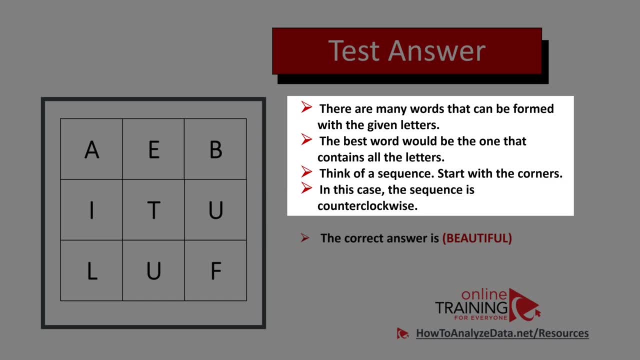 put letters in the opposite orders of the way we currently read this. So, for example, if we read left to right or top to bottom, they might put word letters that will go in the sequence from right to left. 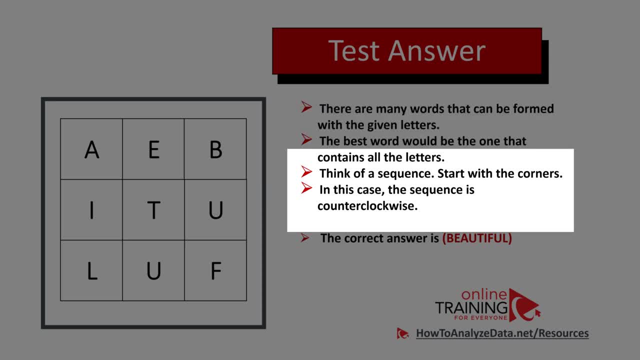 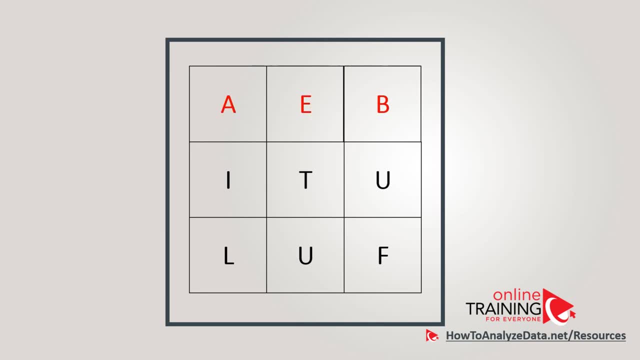 or from to the top, And this is exactly the case here. The correct answer here is word beautiful, which starts in the upper right corner, And then you go by the letters B-E-A, U-T-I, F-U-L. 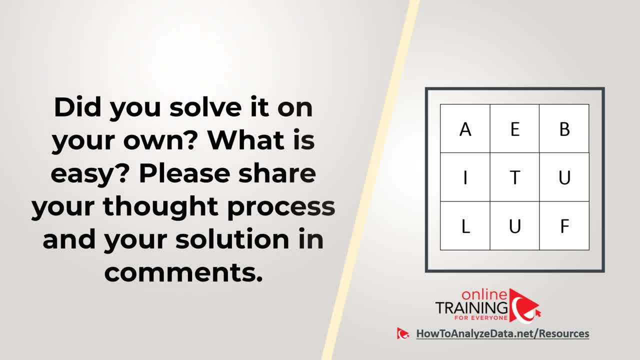 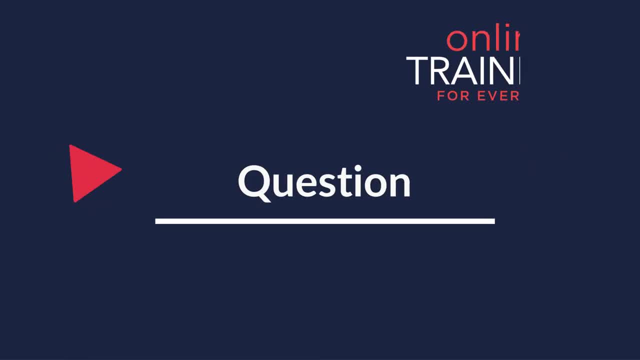 And that's how you get to the correct answer, which is the word beautiful. Hopefully you've nailed this question and now know how to answer similar problems on the test. Here is the very interesting question from the real test. 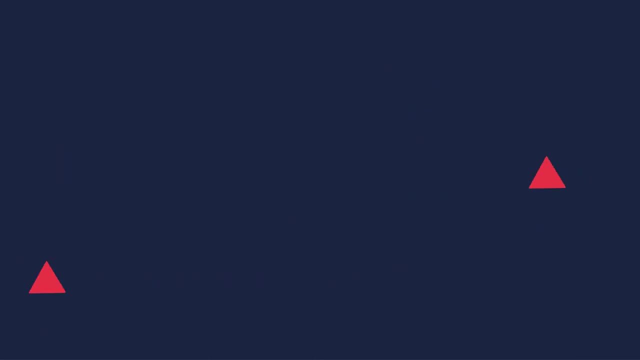 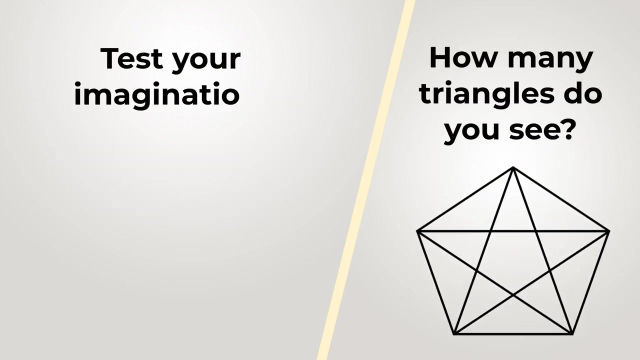 some of you might find challenging. Despite being tricky, you will have a lot of fun trying to find the solution, Because this question tests your imagination, spatial thinking, logical thinking and attention to details. 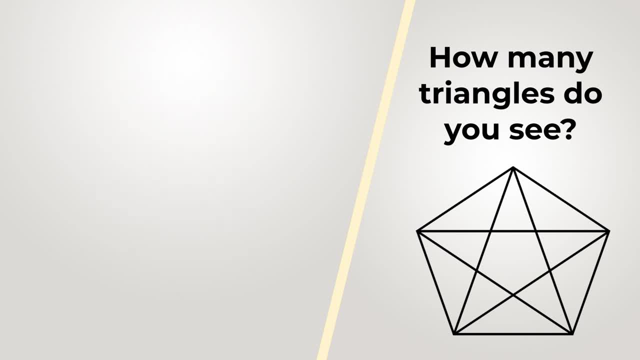 Please take a look at the picture and identify all triangles in this picture. Do you think you know the answer? Now might be the right time to pause this video and see if you can come up with the answer on your own. 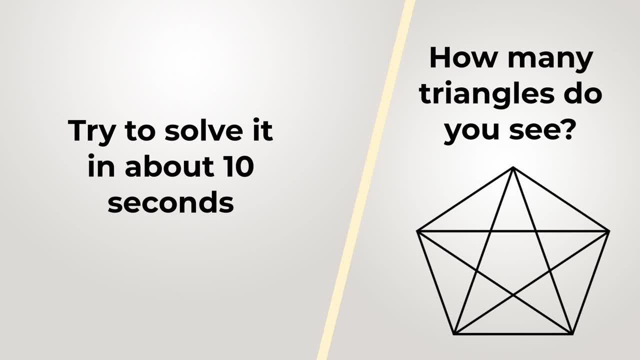 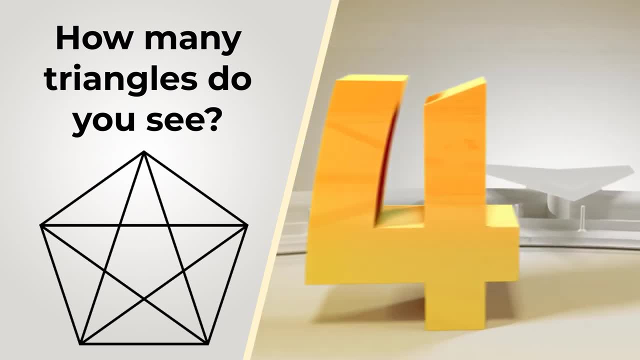 Give yourself about 10 seconds. This is typically about as much time you will get on the real test. Did you come up with the answer? Let me give you a tip. Keep in mind, though, that on the real test, 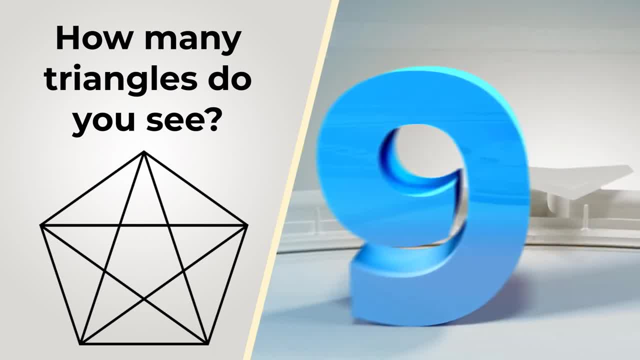 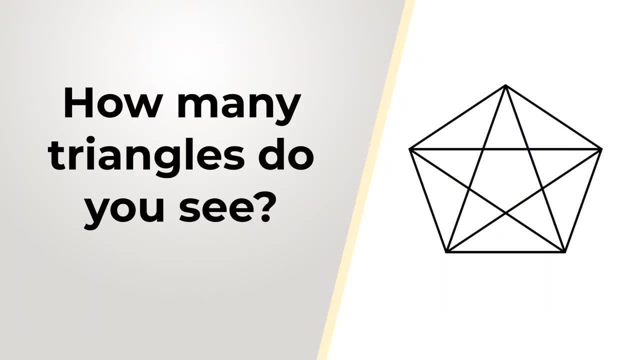 nobody is going to give you any suggestions, But make sure to consider the possibility of one shape being inside the other. Now let's continue to see if we can solve this challenge and get to the correct solution. 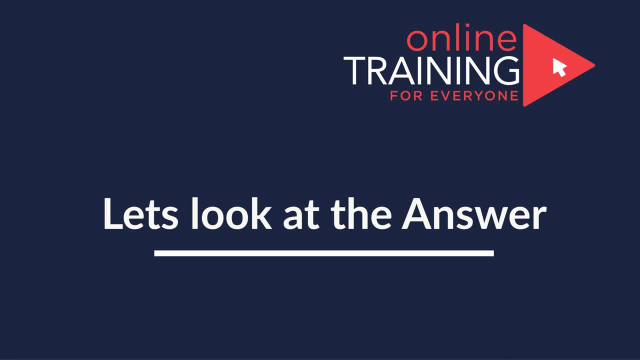 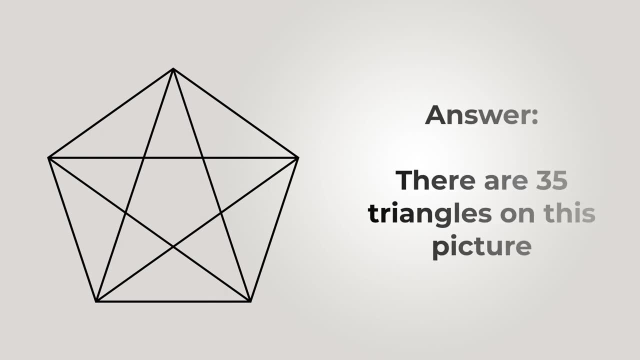 together. It is mind-boggling, but there are 35 triangles here. Can you believe? it Certainly was a huge surprise to me as I was discovering them. Let me draw all of them for you. 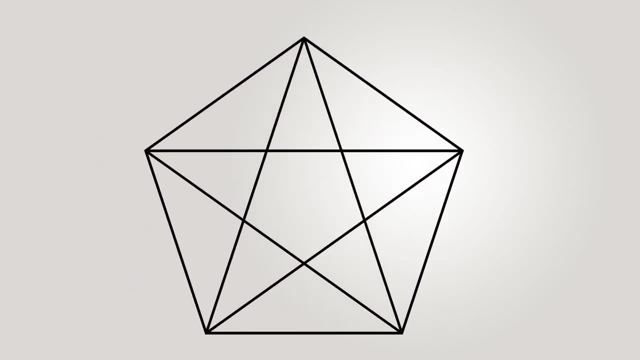 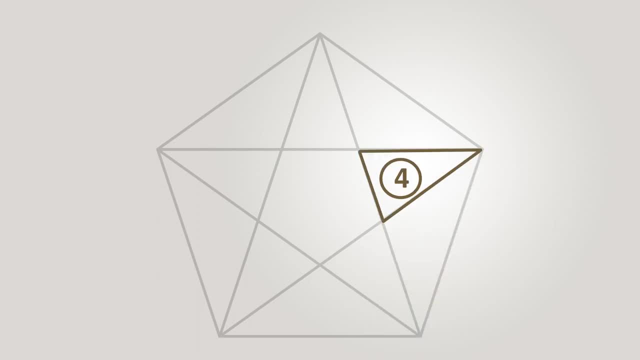 I will start by drawing small border triangles. There are 10 of them. Please count with me: 1..2..3., .4..5., .6..7., .8..9. and 10.. Now let's do. 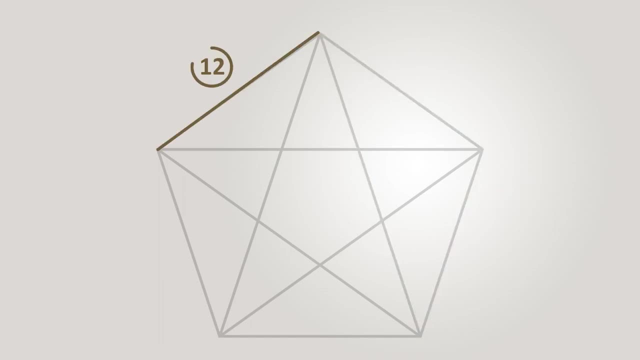 next 10 triangles: 11..12., .13., .14., .15., .16., .17., .18., .19. and 20.. And now let's do next: 5., 22., .23.. 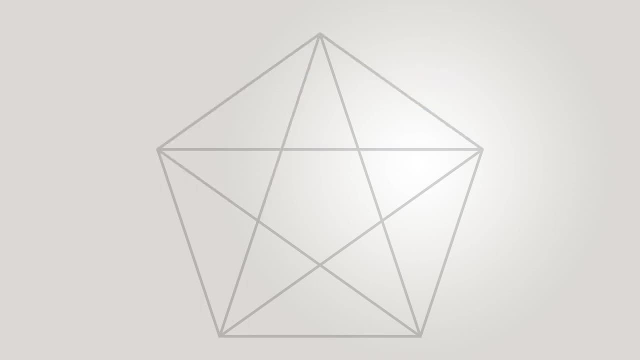 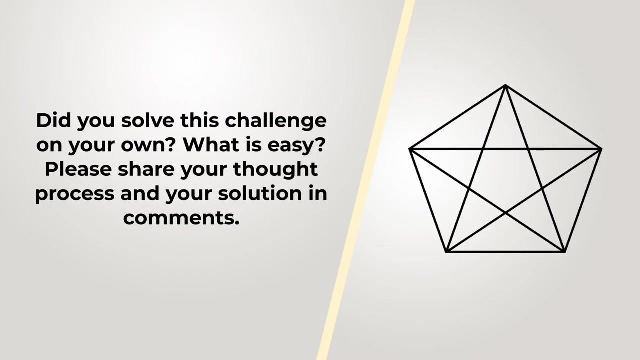 .24.. .25., Another 5. 26. .27., .28., .29., .30.. And then the last, 5. 31.. .32., .33., .34., .35., .36., .37.. .38., .39., .40., .41., .42., .43., .44., .45., .46., .47., .48., .49., .50., .51., .52., .53., .54.. 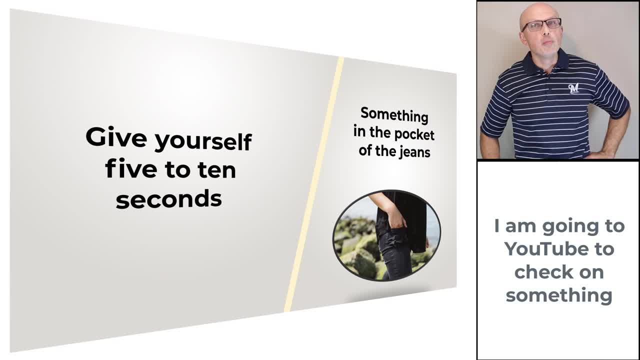 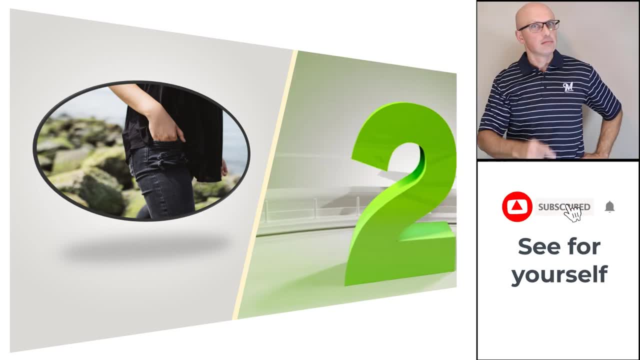 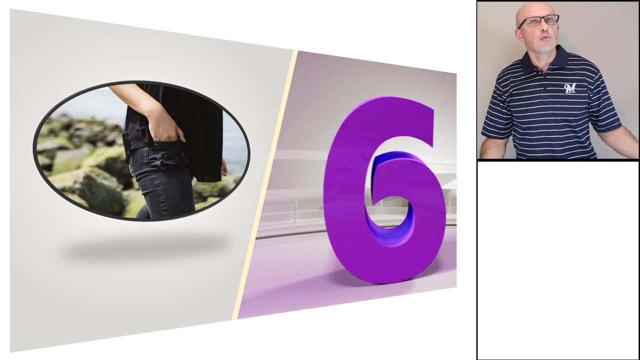 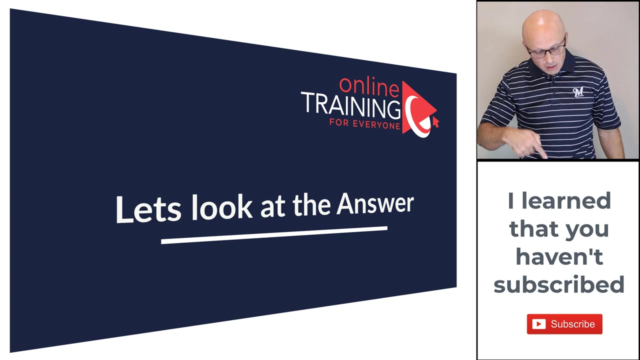 .55., .55., .56., .57., .59., .60., .65. .66.. to see how we can solve this challenge and get to the correct solution together. And the solution is very simple: There was a hole in the pocket of the young professional's jeans. 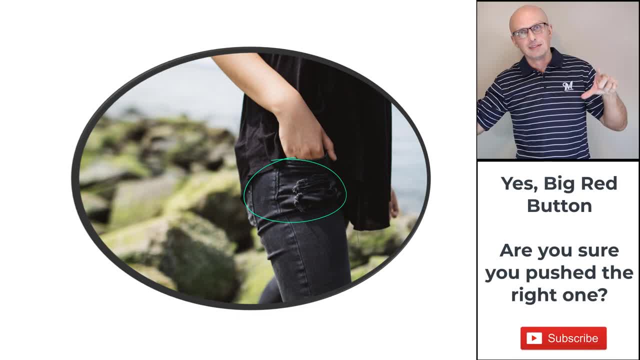 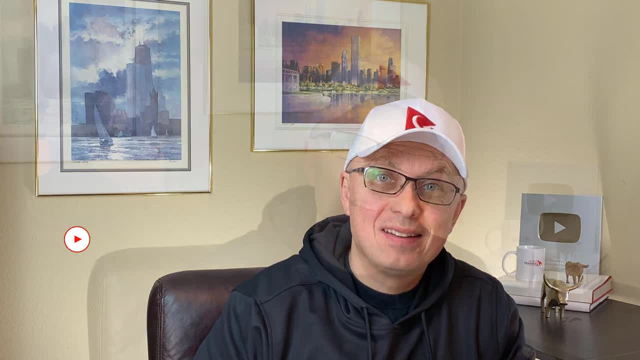 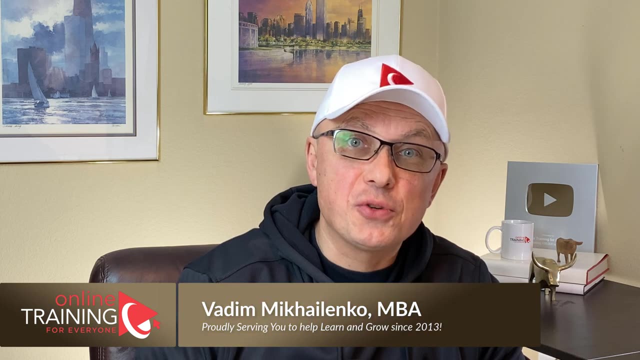 Hopefully you've nailed this question and now know how to answer similar problems in the test. Thanks for watching. If you liked the content, please give us a like and consider subscribing. Thank you for your endorsement, support and patronage. Please also check out additional resources in the description section of this video.